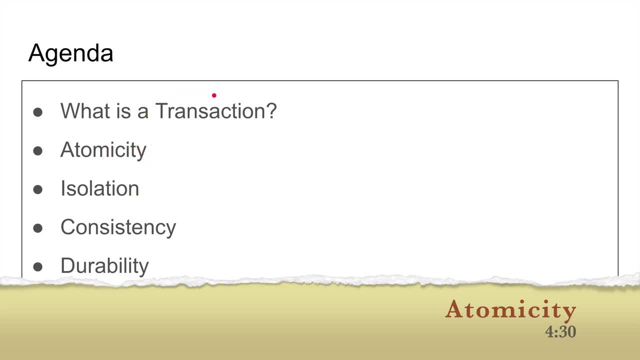 through a transaction. we're gonna talk about atomicity. I flipped the two properties, isolation and consistency, so it's acid but I a slid. I changed it because there's a reason. talking about isolation will- and it doesn't have a Thomas T will- lead to consistency in a very nice way you're gonna talk about. 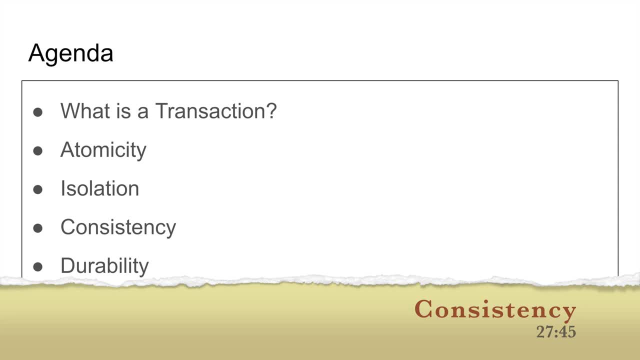 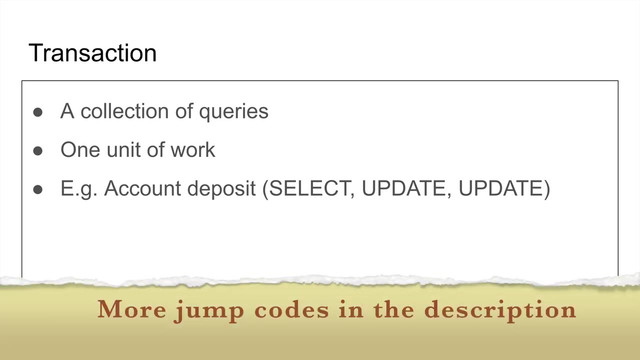 consistency. I talk about a little bit of a no sequel, databases, why people are moving to a no sequel, why they create a no sequel. to begin with, okay, and then, fourth, we gotta talk about durability. just kind of very straightforward thing, right, transaction. what is a transaction? we hear this a lot in databases: a. 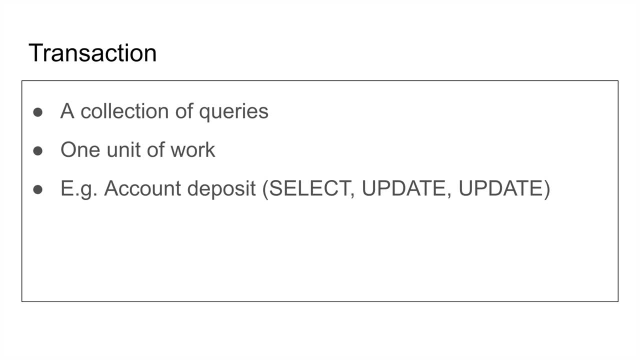 transaction. it's nothing but a bunch of queries, okay, it's a collection of queries, so it's a one or more queries, okay, and that property of these queries or they, are you one unit of work? an example would be: if you want to deposit an action account, right, and if some cash into an account, that is actually a select. 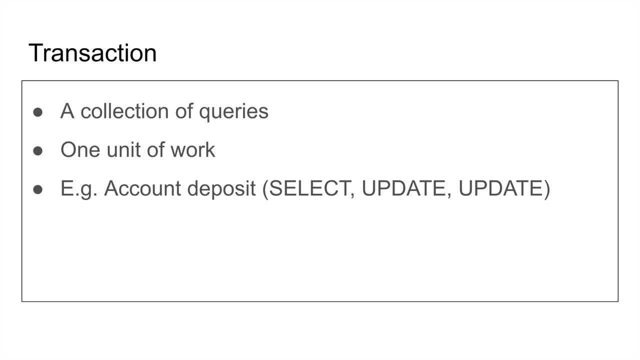 statement, followed by update statement, followed by another update, seven, like we we're gonna show in a second right, but each one of those is a query. the three of them can form a transaction and you define what a transaction begin and where transaction end, and we also. there is another semantic attached, a. 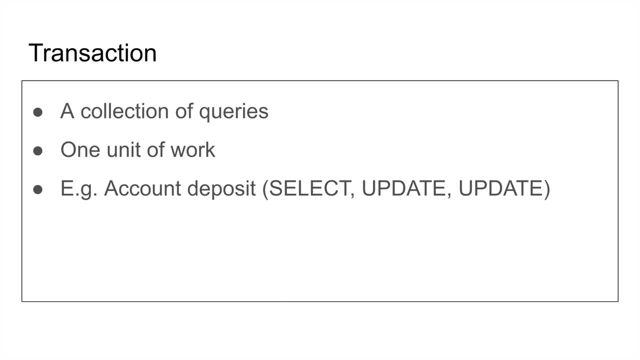 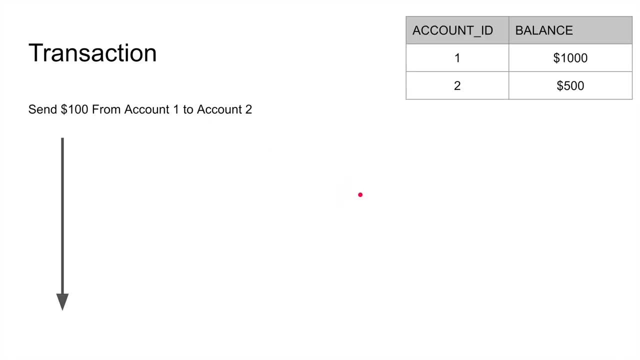 let's just jump into example him a transaction. I have an account here with a beautiful table, just to feel, because that's all what you need obviously for in a bank, right? just two fields account. you don't need a name, you don't need anything else, no date, nothing else. don't need it, don't need anything else, nothing else. don't need it, don't need anything else. 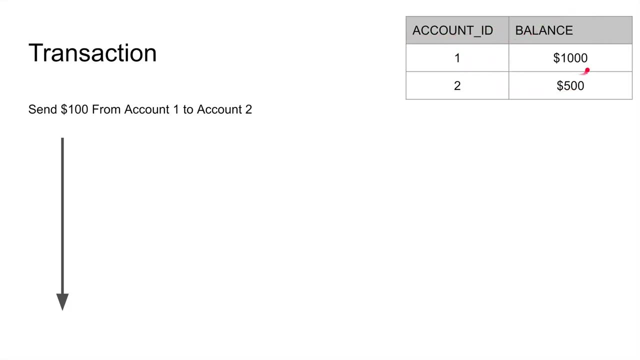 just to feel so. there's a count ID, there's a balance. this guy has a thousand dollars, guys had a two, five, five hundred, and the transaction is send hundred dollars from account one to account two. so what do we need to do first? does account one even have a hundred dollar? I don't know. so I need to. 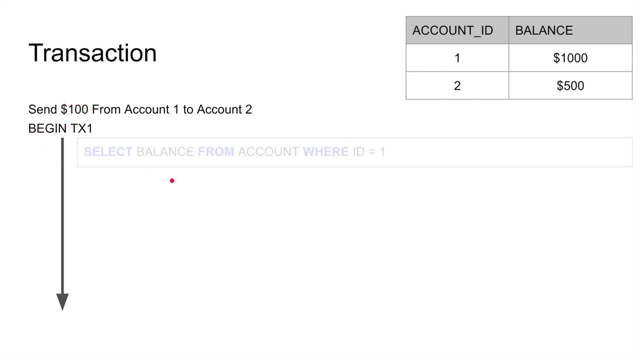 check. right, so that's, we're gonna begin the transaction. get a select, let's check the balance. do you have a hundred dollars, sir? yes, your balance is play a balance greater than 100. yeah, sir, it is greater than 100. all right, let's debit that hundred minus hundred, okay. so now it's 900, okay, but that's not. 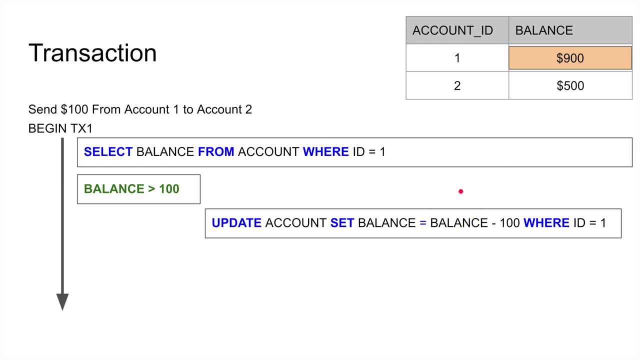 committed. yes, just yeah, meh right, it's just touched, it's a dirty change, okay. and then I'm gonna add another hundred to the second account, gonna commit my changes. turning green: that means it's like it's presented, all good, we're happy and that's it okay. so that's essentially. 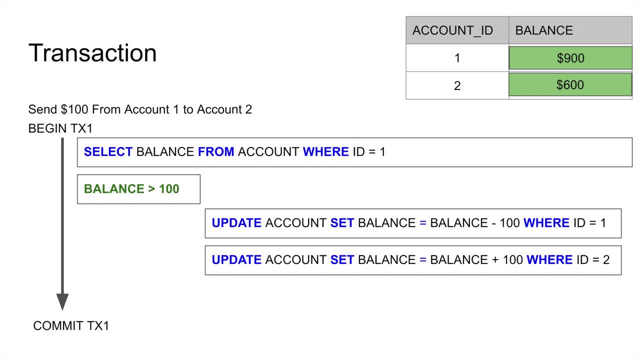 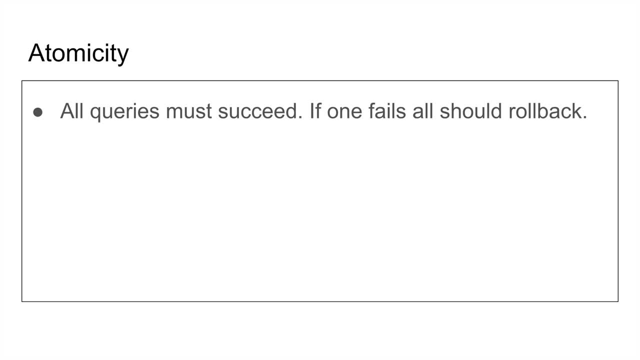 what a transaction is. it's a unit of work, but it consists of multiple queries, one or more. okay, that's a transaction. let's talk about the first property, now that we understand transaction: atomocity. atomocity is came from the word atom, right in science. where is an atom is the smallest piece? 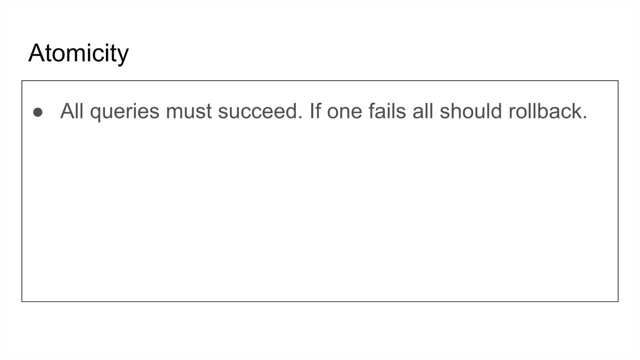 of a unit that cannot be divided. you can divide an atom unless you're doing a nuclear fission and all that stuff. but let's assume atomic atom cannot be divided, can't be split, and that's what a transaction is here. a transaction should be atomic. when we say a transaction is 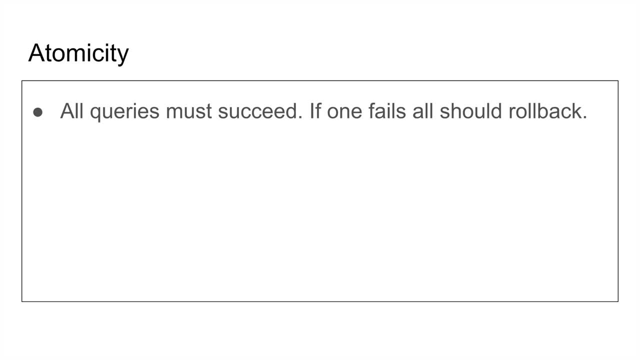 atomic. that means all of those queries should succeed, and if one of them fail, you better fail the whole thing, you better roll back the whole thing. and now we know what a rollback is. does that make sense, guys? very simple concept, and just tell me why it happens. okay, why does it matter, though? why does it matter? 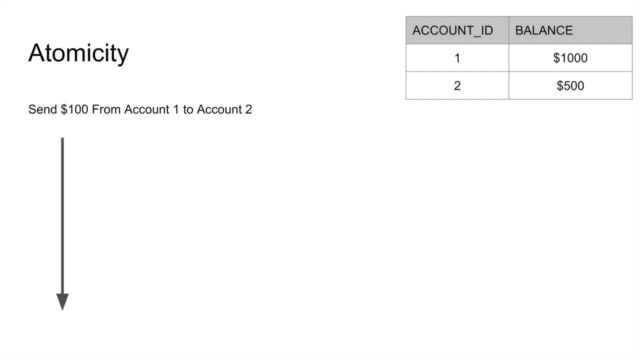 why should I care? okay, why are you enforcing that? well, where you gonna know, sir, they're the same example without algo insidi, let's say, I don't have it almost city, I don't enforce this in my database. well, there's the vendor of this database, Oracle, Postgres. didn't I implemented, although must do, which is 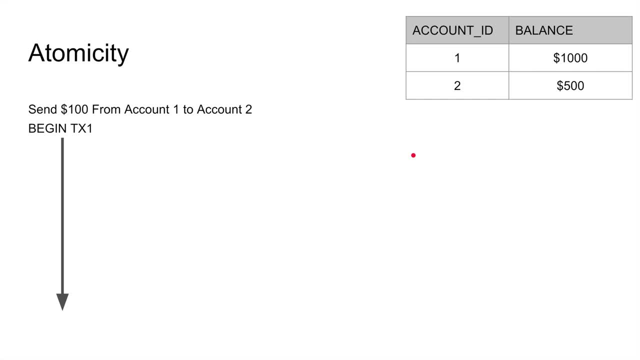 bad. all old relational should implement intimacy. let's say I'm gonna deposit the same time's lecture. I'm gonna do it, but we're gonna add some a little bit spices. let's say I'm gonna deposit the same transaction. I'm gonna do it, but we're 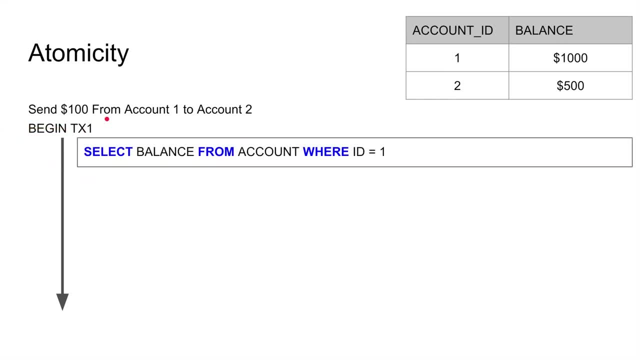 gonna add some will be spices on the Nephilim and all this stuff. like a top of that, again there's action. I'm gonna dip it. hundreds of code- okay, I need to check this. this guy have a hundred. he does, sir. okay, cool, go ahead. 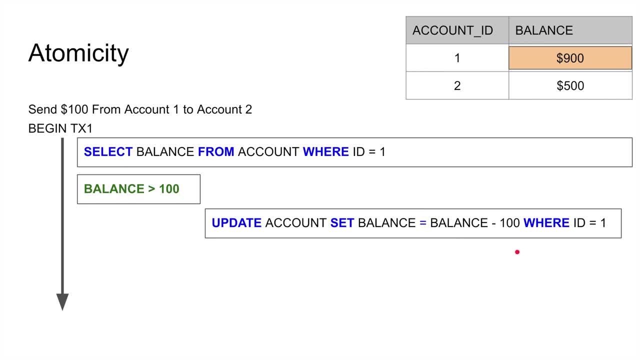 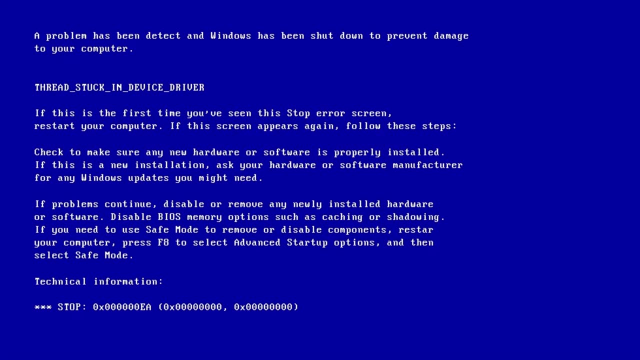 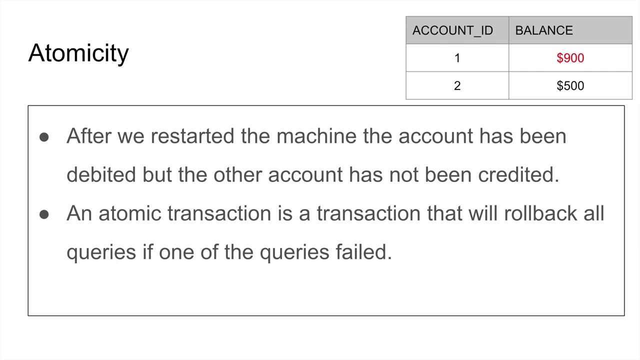 and dip it back out right with a hundred. and what the heck happened? that's not my machine, that's just a slide, guys. but yeah, your database crashed. something happened. you went back, restarted the database. guess what? that's the last thing you did. you, you dip it in one account by you for, but you didn't get to the other. 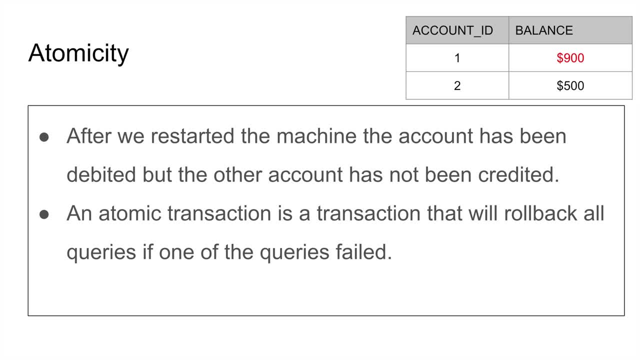 part of the transaction to actually commit and change that to six hundred. so now you have a hundred dollars in the thin air. it just went away. all right, that's just bad ish. right, that's very bad ish. okay, after we restarted the machines account to get credit, obviously. so that's what a Thomas. 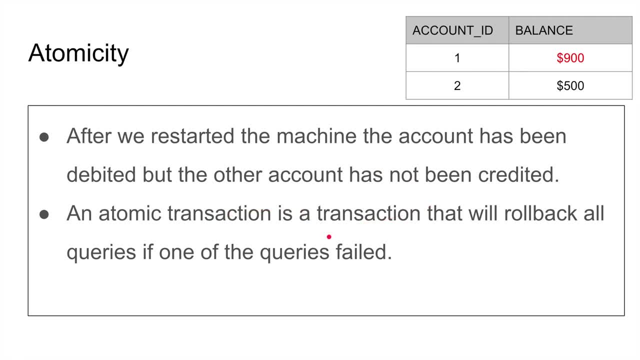 transaction is a transaction that will roll back all queries, all changes if one of the queries fail. so that's what it means essentially, right. so if this is what we had just did is not atomic transaction, what happened is is bad, right. so the correct way is to just roll back and roll back this 2000 does that? 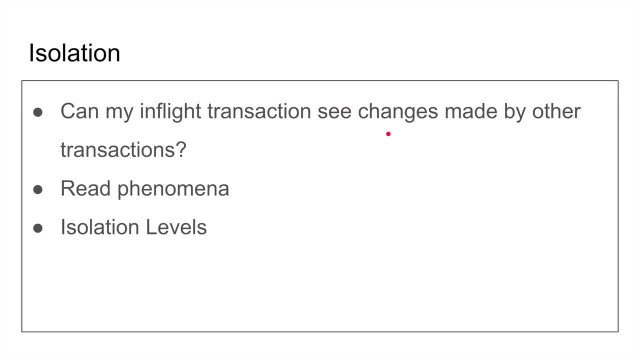 make sense, guys. that's what an atomicity is. very simple stuff. jump to the second one: isolation. I skipped consistency because we're gonna go back to consistency and later, after isolation. this is one of the longest and, in my opinion, one of the most critical properties a software engineer really should understand. really. 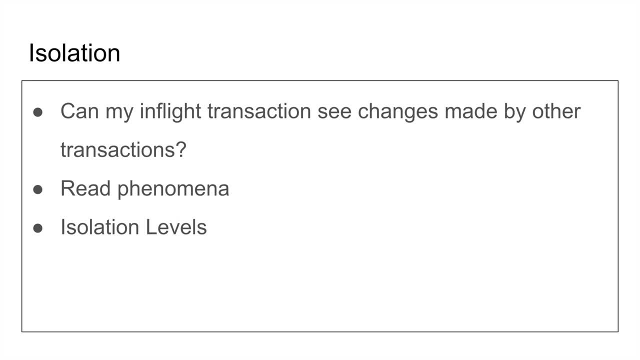 should understand isolation. what is isolation- and isolation is to be isolated- is I want to stay alone and I don't interact with the world, right, okay, let's take this in the transaction. a transaction is to have a transaction that is later. that means, and in flight rise as a while I'm executing a transaction. can this transaction see? 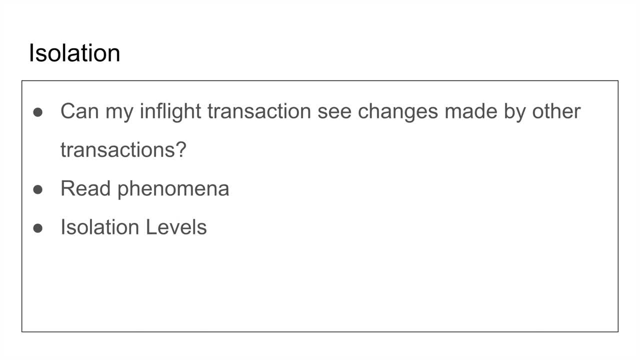 other changes made by other transactions and there are in flights. okay, so that's what it means. I am now executing my stuff. can I see other stuff people are making? okay, and is that okay? right, and my isolate from the other world? okay, and, And it's really up to the implementer, the software engineer here, to adjust this knob of isolation that we're going to talk about. 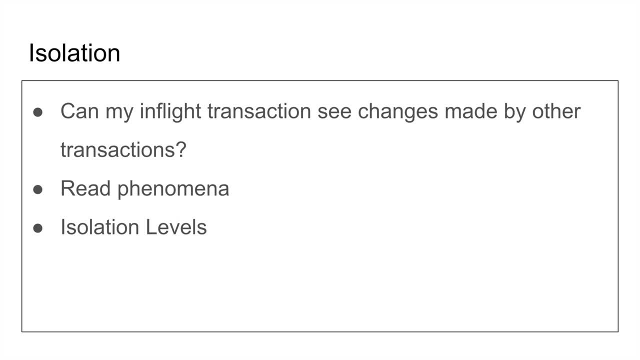 Do you want no isolation? I don't care, You can change anything you want and I'm going to read whatever you change and that's maybe okay, But some cases it is no. no, sir, We're going to talk about that's isolation. 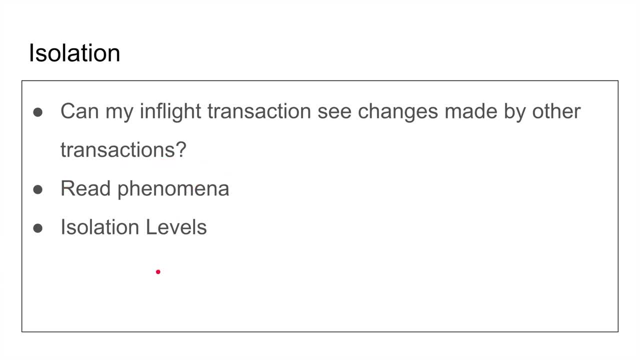 We're going to talk about as a lack of isolation. you're going to get these read phenomena. I don't know, it has a fancy name. for some reason. You're going to get some read ugliness, read weirdness, some weird stuff, while you're reading transactions. 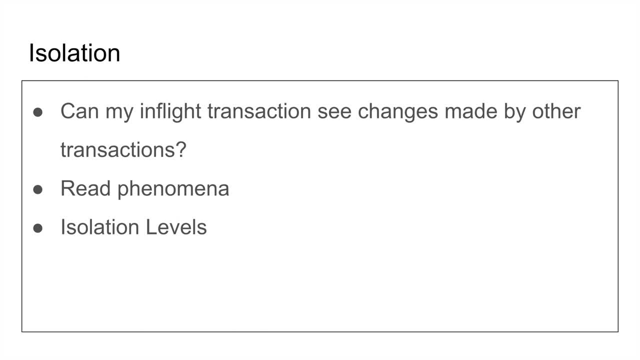 And as a lack of isolation, we're going to talk about that read phenomena- This is dirty read, All that stuff- And we're going to talk about isolation levels that a database can implement to get rid of the read phenomena. So without isolation, you get a bunch of read phenomena. 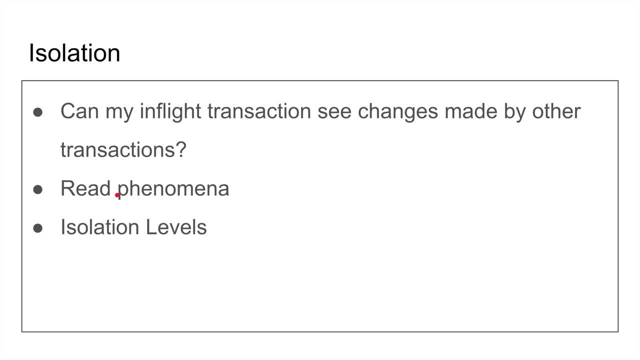 We implement isolation levels to fix those problems. Let's talk about them. Let's talk about the read phenomena. We have three. I added the fourth one. I don't think It's a read phenomena. It's one of the bad things that can happen as a side effect. but I added it anyway. 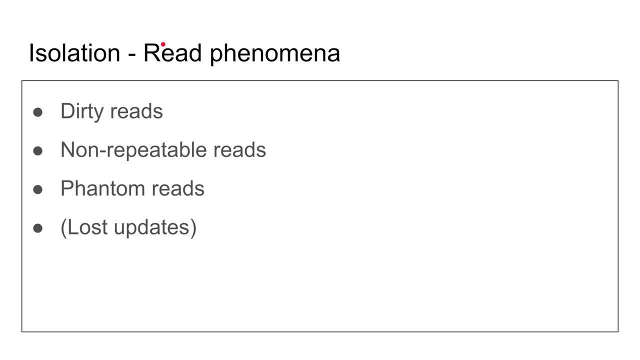 Okay, So the first one dirty read. There are two reads. essentially is: I am And we saw that right. I don't think we saw that. Yeah, But essentially dirty read. What it is essentially is like I am in flight transaction and some other transaction made a change. that transaction did not commit that change. 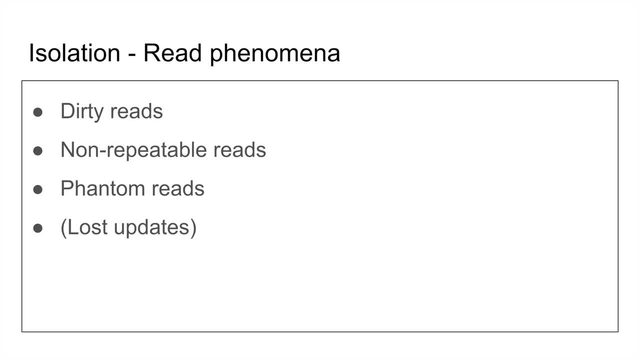 And I read that change- Okay, So any minute that transaction can roll back that change- and I just read a bad value, a dirty value that hasn't been committed. That's what it means essentially: Non-repeatable reads. We're going to talk about that. 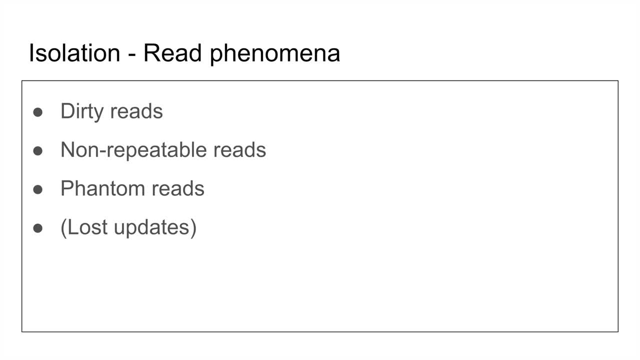 It's like I read a value that is being committed- right, Not necessarily committed or not Okay. But then I turn around and my same transaction and I read the same value, whether the same query or other query that give me the same path to that value. 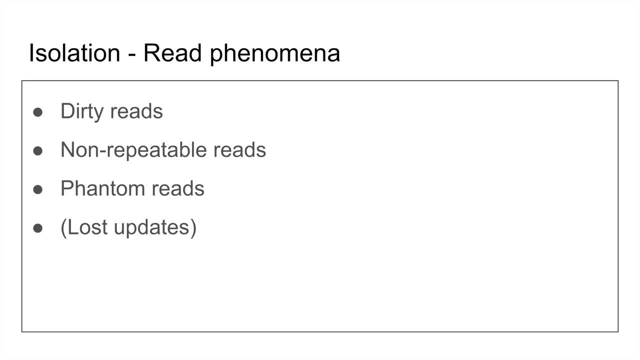 Okay, Like a range query, And I did not get the same result. So my results, my reads, were not repeatable in my same transaction. Some some users are fine with that. Some users are not fine with that. We're going to talk about that. 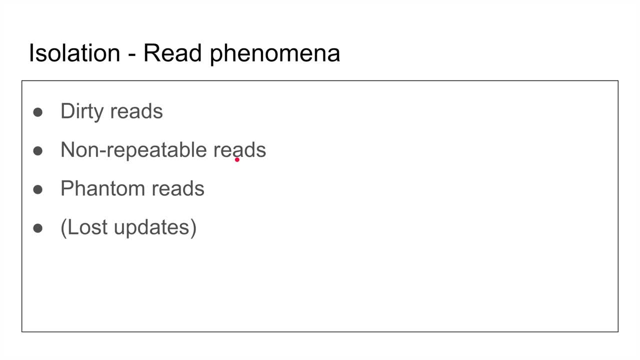 Okay, Phantom reads: I inserted a new, another transaction, inserted a new record and I picked that up where I shouldn't have picked that up. Okay, It's usually happens with um Range queries: lost updates is like when when you're started to change something right. 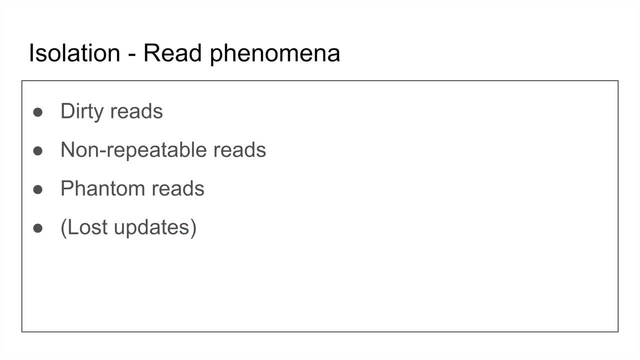 You changed in the transaction. you change the value and some other transaction overwrote your value before you even committed, So you're going to commit a wrong value, So you just lost your update. essentially Okay, And uh, these are the four phenomenas. 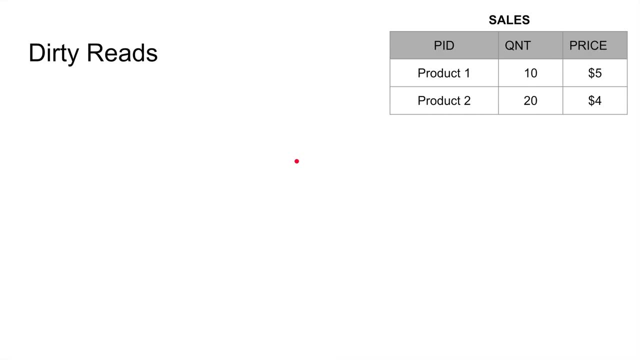 Let's talk about each of one. one of them: Read dirty reads. Let's talk about dirty reads. So we're talking about it. Read it, Or dirty reads. I am going to read a value that hasn't been committed by another transaction. 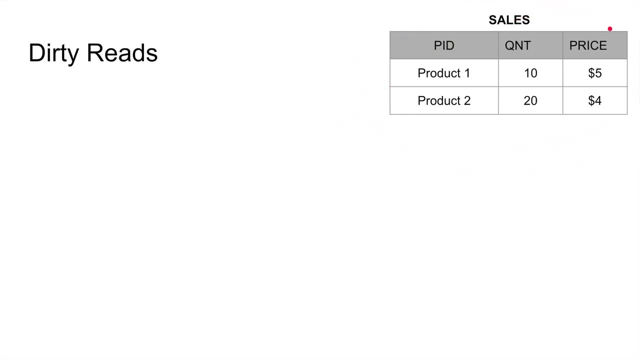 Let's see. I have a sales table here. There's a two products: product one, product two. There's a quantity of sales. This product one has sold 10 units at a price of $5 product to 20 at a price of four. 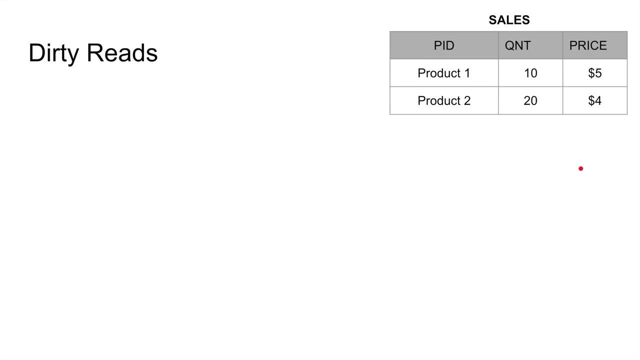 And I am asked to write a query to produce a report of my sales. So what I'm going to do is select the entire thing And some of those Guys- so product one has sold what $50 product to, has give us like $80. 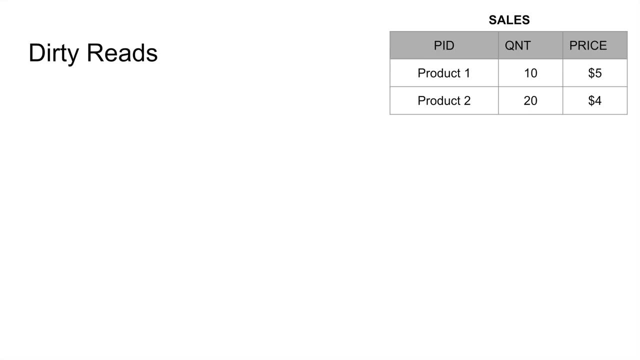 And then at the end I'm going to just view the sum of all the sales. Okay, Very simple stuff. So to do that they're getting a transaction. Okay, Even if we don't really need to commit or change, you can also begin a transaction, right? 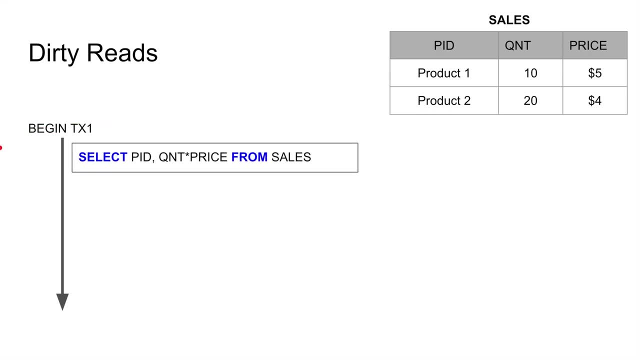 And that's and that can have its values. I'm going to begin a transaction selecting the product ID and then multiplying the quantity times. Okay, So the price obviously, and then from sales. that will give me what we just saw, right. 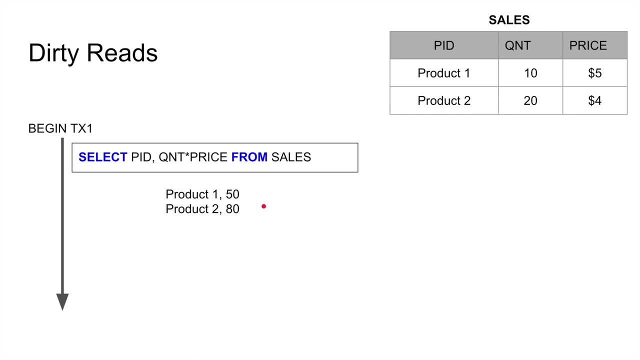 Product one: 50. product two: That sounds good, but here's the trick: while this is executing, another transaction, just begin right And this talk another quantity. it just added some some. someone made us another sale right And they updated the sales report. 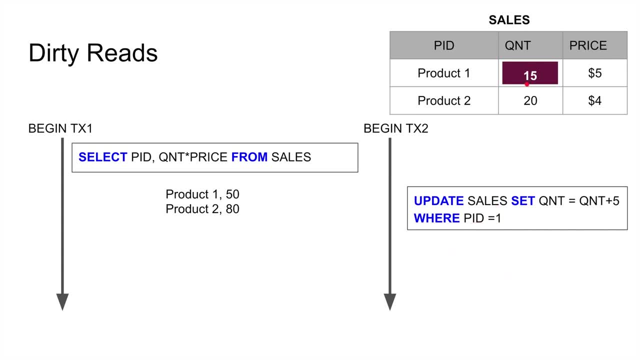 Okay, Where the PID is equal one. So now we just increase the quantity, We buy five. That's pretty good, but I don't know if it's good because we just read this Now. I just have an old value and might be that 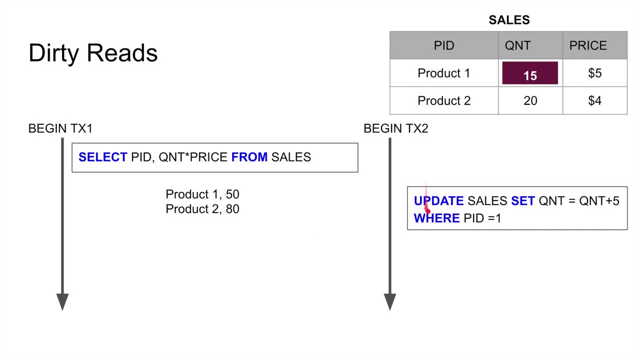 Okay, But let's see what will happen, Right? So I didn't commit this transaction to yet, right? While I'm doing that, I did the second query, which is select some quantity times price, which is literally this times this plus some 20 plus four. 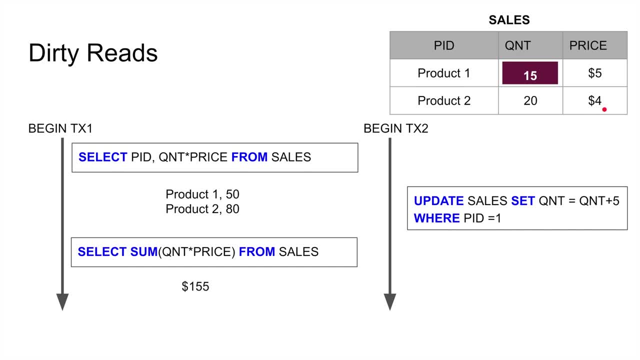 It was guess what. this is giving me a wrong result. This is now reading the dirty value that never been committed. yet This guy's reading it, and that's a dirty read, right, We're reading the bad value. Why? Because it's leading to a bad result. 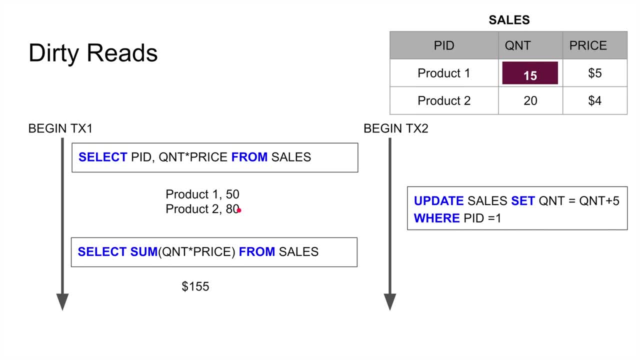 See: 50 plus eight is one 30, but I am showing the report, one 55.. So you can See dirty reads are bad. Okay, I'm not saying they are always bad. It's up to you if you can tolerate that or not. 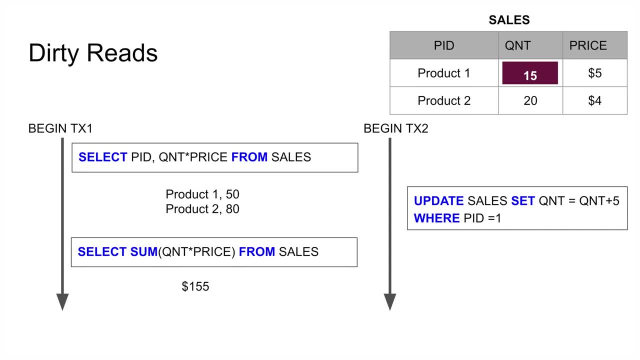 If you're building Instagram, for example, you don't really care if the number of likes doesn't match the number of user who actually liked the picture right, So you, you might. there's a price for everything, Guys. we're going to talk about that. 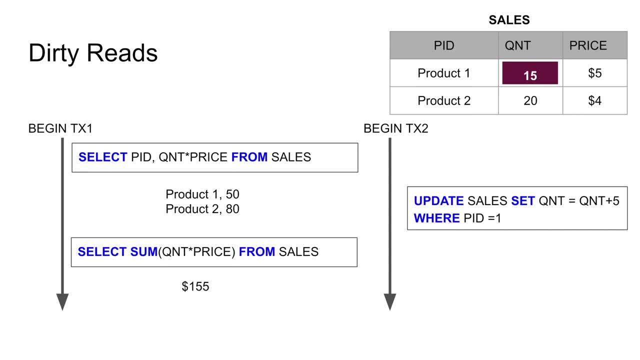 Okay, This is. you cannot just say, yeah, I'm going to implement the best isolation ever again. So there's three First Read phenomenon: Okay, And we commit that transaction, obviously, but it's, it's useless, We got bad results. 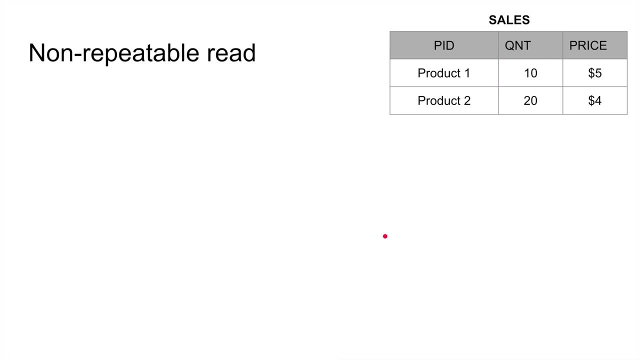 So that's dirty Read. Let's talk about non-repeatable read. Okay, A non-repeatable read is, as we said, read that I'm going to read something in my transaction and I'm going to read it again. I'm getting two different values. 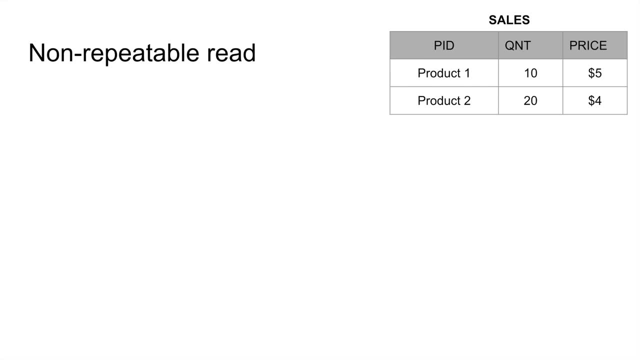 You might say: why are you reading the same values twice? Are you idiot? Why are you doing that? You just read it. Why are you reading twice? There are, believe me, when you're writing code, when you're writing transaction, you 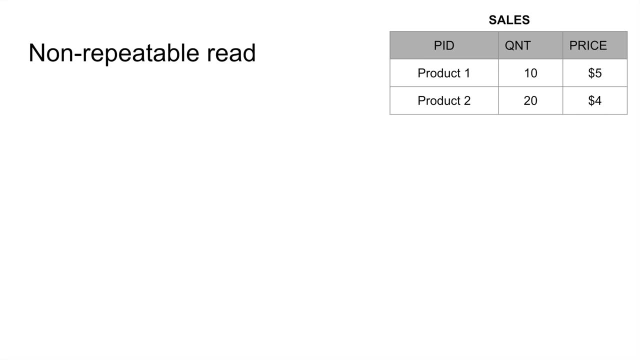 will need to do that sometimes. Okay, And we're going to show you an example. Okay, I had to think about an example of this, but here's an example. same thing right. Beginning the transaction, I'm going to select the count of report, right? 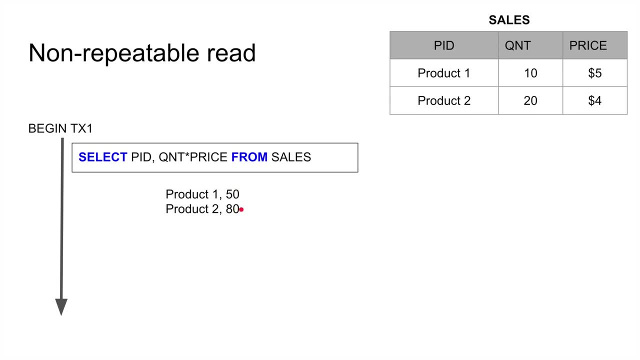 That sounds good: 50 and 80,, right, And then, uh, this is, the total of this is one, 30,. but guess what? A transaction began at the same time and it updated the count. It sounds like it's the same transaction, but here's the little bit different. 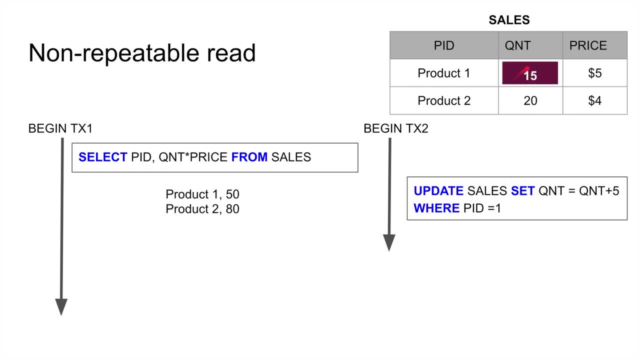 I did here. I actually changed that. Okay, Now it's 15 and I also committed. That's the difference between the first one and that. So whatever I'm doing next is actually not a dirty read, right? I'm reading a committed value. 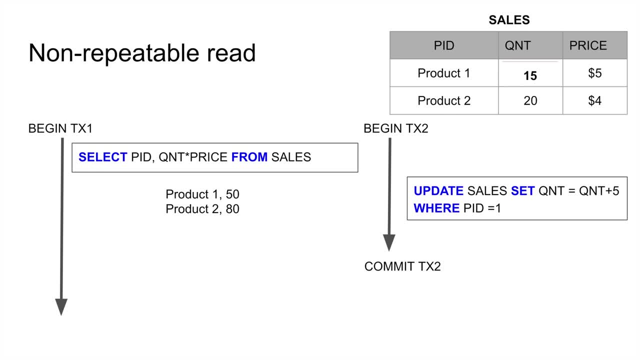 It's a legit value. but the question is, should I read that committed value or not? Okay, So to me this has been committed, It's a legit value. It's not like the previous one where someone actually rolled back right. 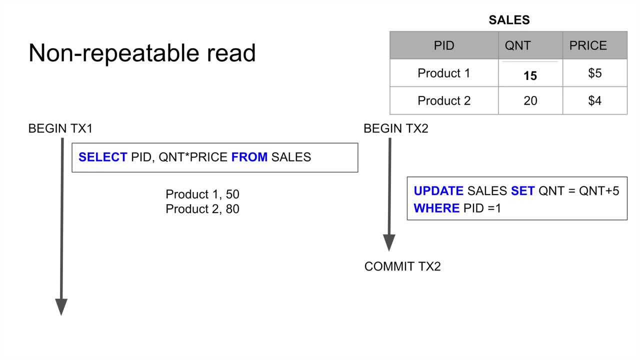 Or or it could could be rolled back. It's not a dirty value, It's an actual committed value. So I'm going to turn around, do the sum, but now I'm going to get a bad result. Despite me committing, I get a bad result. 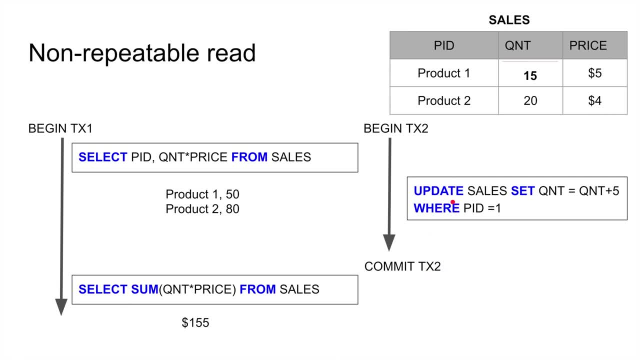 So having it committed or not doesn't really matter. Now I got this phenomenon of a non-repeatable read In this example Because their first read gave me that sum 130.. The second read gave me a different sum. Okay, 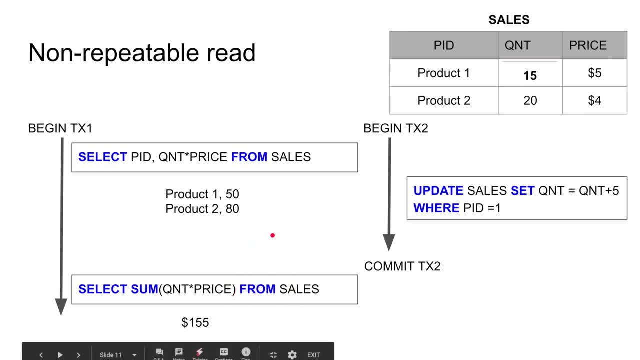 So that's a non-repeatable read in itself. Okay, A non-repeatable read. So we read this first, we get a result. Then we read it again, We got a different result. So that's a non-repeatable read. 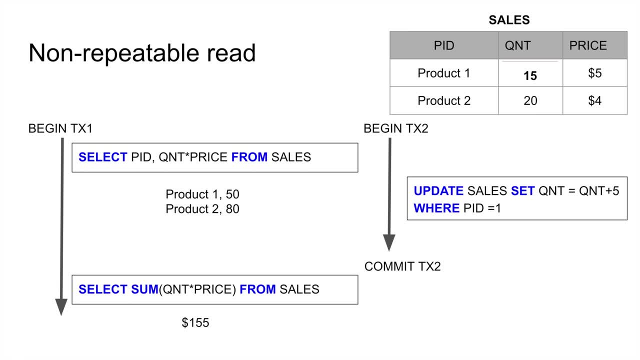 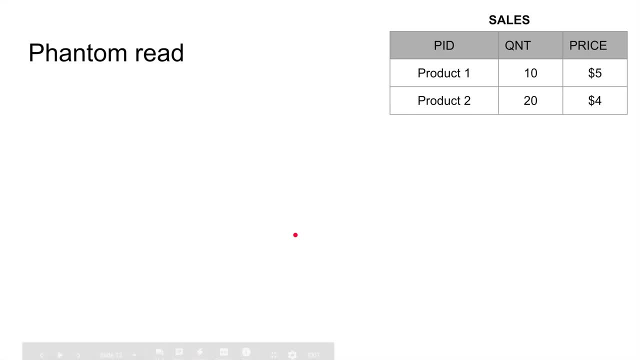 We're going to discuss ways to fix this right. How can you fix this? We can talk about things. how to fix that. Okay, Non-repeatable read, right, And obviously you're going to commit at the end: Phantom read, phantom reads. 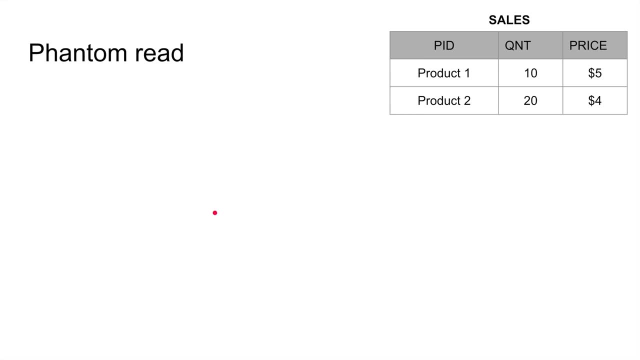 So what phantom reads is actually interesting, because here's an example of phantom reads. right, Let's say I begin a transaction, do the same thing, select the account and then sum the whole thing. We get 130, 50 sales and 80, right. 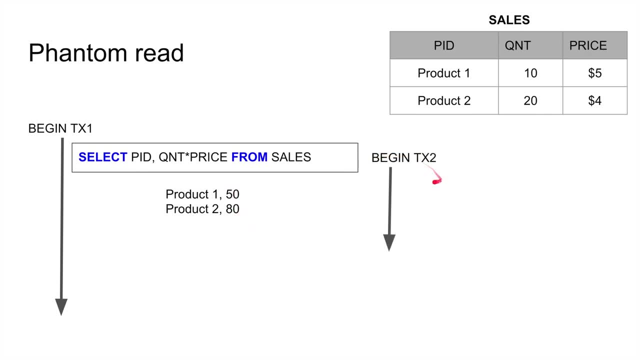 At the same time. here's the other transaction. It didn't actually update, it just inserted record. It just inserted a new sale of a totally different product And now, as you've noticed, the new sale, the new sale. You committed that, so it's changed. it's in the database. 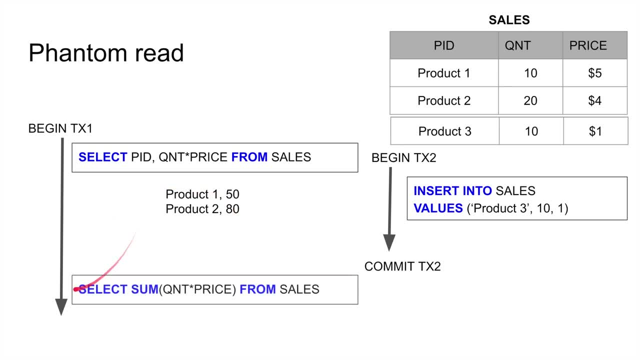 And in the same time the first transaction is still executing. I am selecting all the count prices from sales. That is bad son, Because now you just accounted for product three on the first sheet of your paper report. you did not account for that right. 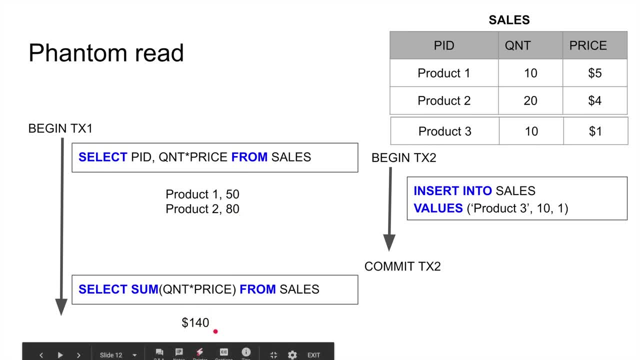 So now the sum of those obviously 130, but you showing 140,. okay, That's a phantom rate. and the reason it's phantom rate? because this is one of the range queries where you're selecting but you're getting extra rows. 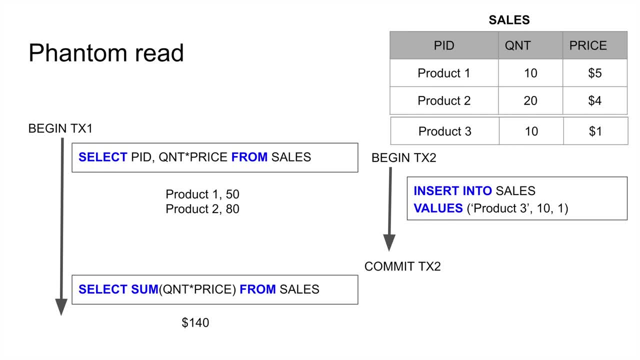 So if we're gonna talk about ways to fix that, this is a little bit harder to fix and to avoid The previous ones, you can implement locks and version controls to get away with it. But this, this is a new value. how do you lock it? 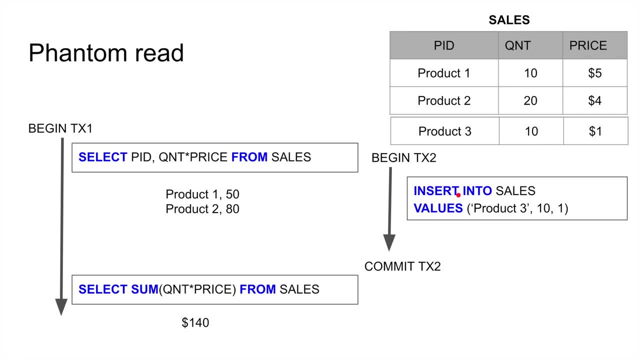 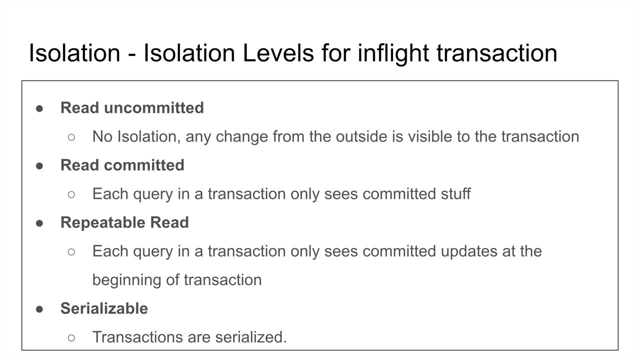 It's a new value. you cannot say, hey, don't read that, It's just really interesting. and one of the ways to fix that is actually serialization. isolation level. Let's talk about the isolation levels, right? This is very interesting guys. I really like this topic. 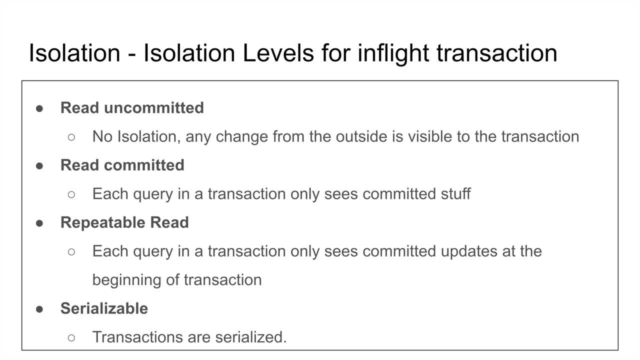 So isolation levels are levels, Levels of isolation, duh Hossein, what are you talking about? So isolation levels are levels that are implemented by the database to fix those phenomena that we talked about. okay, And there's a nice table by Wikipedia here. 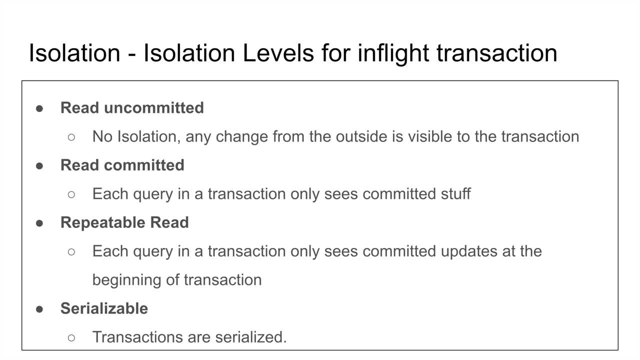 that I'm gonna reference here. it's very nice. It just explains the whole thing here, okay. So read: committed is the first type of isolation, which is- I don't know why I call it isolation level. It literally offers no isolation whatsoever. 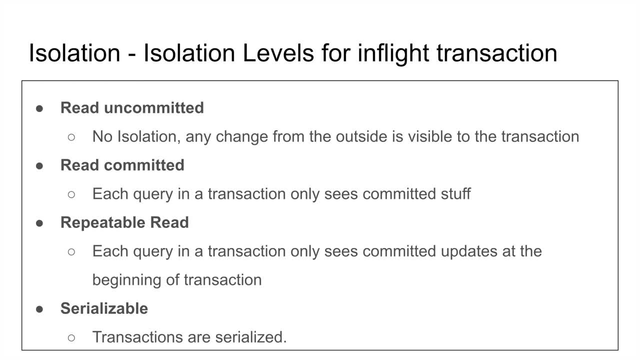 That transaction. when you open it, you can see. okay, when your transaction starts in a read uncommitted way, it's not gonna perform any isolation. Any changes to the database is happening. you're gonna see it. So you're gonna get dirty reads here obviously. 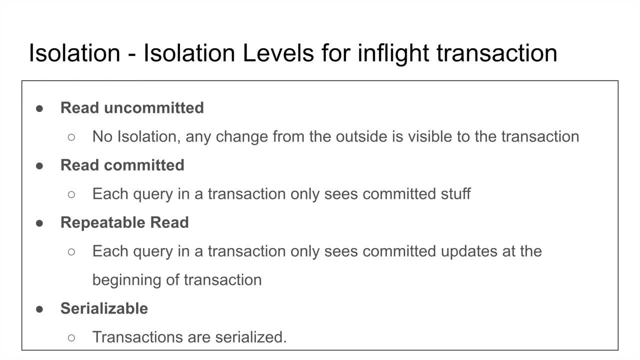 because you're just cheating everything. You're gonna get non-repeatable reads. obviously. You're gonna get phantom reads right And you're gonna get lost updates as well. yeah, The read committed is each. there is a little bit of isolation. 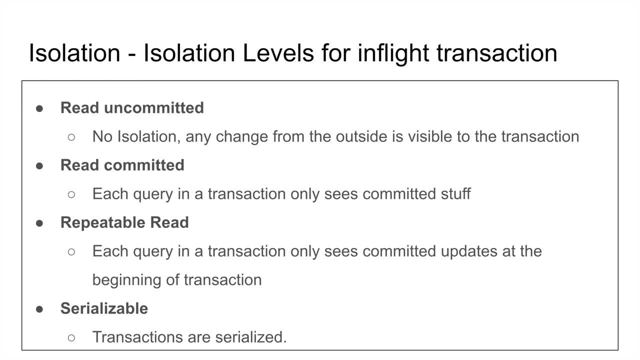 here and most databases implement that okay And most of the time this is one of the best transaction isolation level, because you're happy with that. You're happy to read committed stuff. But here's the thing: Each query in the transaction only sees committed stuff. 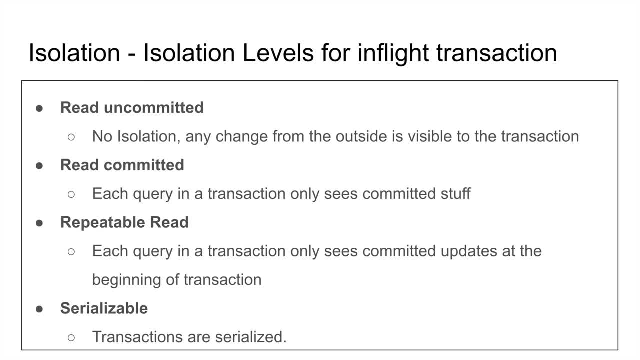 at that time of the query. So each query you execute gonna see the new committed values at that time. okay, And that could be fine, right? Sometimes it is not okay. So that's what it means: the read committed, You are seeing and viewing the committed stuff. 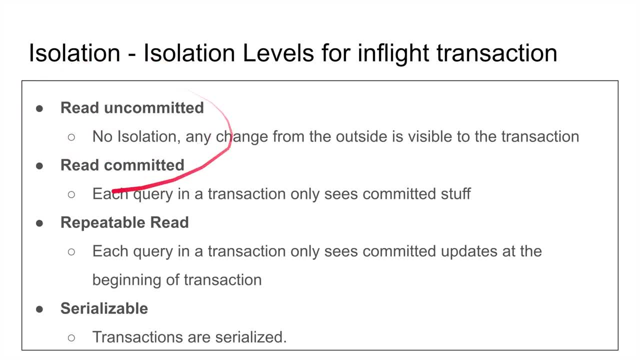 at the time of the query. okay. So anything that is committed, you're gonna see it okay. Obviously, this does not work on our example that we showed. because we showed even that is committed, the sales report came out wrong, right. 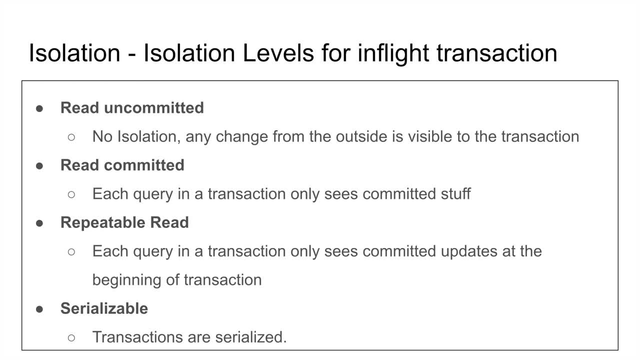 But there are certain cases where read committed is enough for you. okay, Repeatable read. each query in the transaction only sees committed updates at the beginning of the transaction. So the repeatable read- isolation level gives you the ability to see committed values, but not at every single. 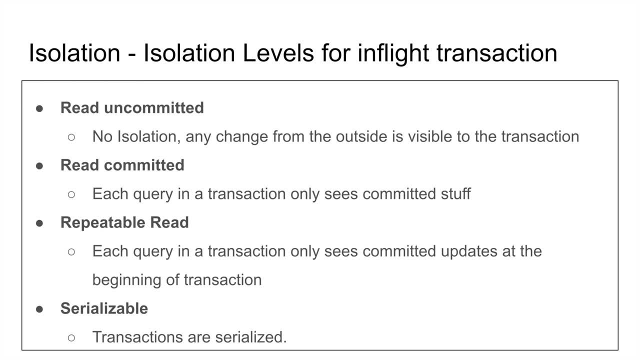 query at the beginning of the transaction. So once you begin a transaction, you will only see changes that have been committed before you started the transaction. Okay, So that gives you a nice isolation, tied to view, and that's really powerful stuff. So now I'm not gonna go through the implementation aspects. 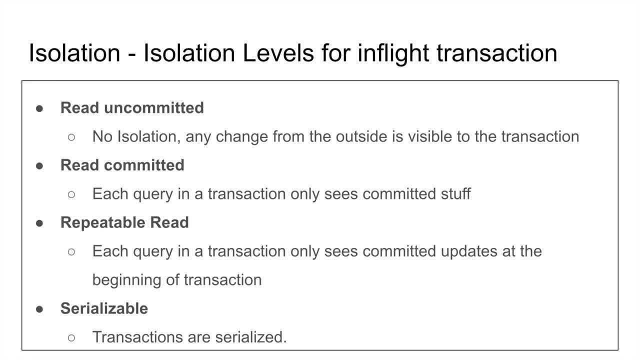 of this databases, some databases implements versioning. to implement this, like hey, when you start a transaction, like Cassandra, right, You start a transaction, I am in version zero, okay, And then anything I read belongs to version zero. 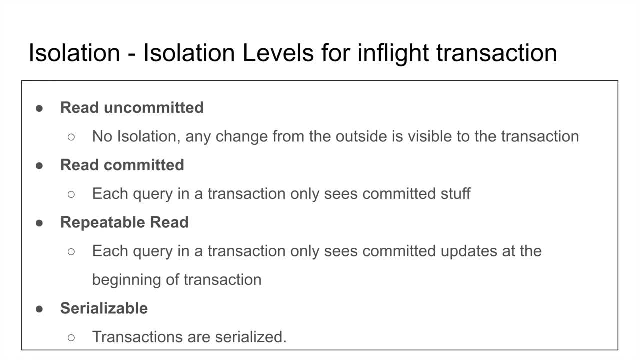 of the database. okay, So if other transactions are committing stuff, changing stuff, they are updating to version one or version two or version three. I am only reading version zero And that gives me a nice consistent view which we're gonna talk about. that right. 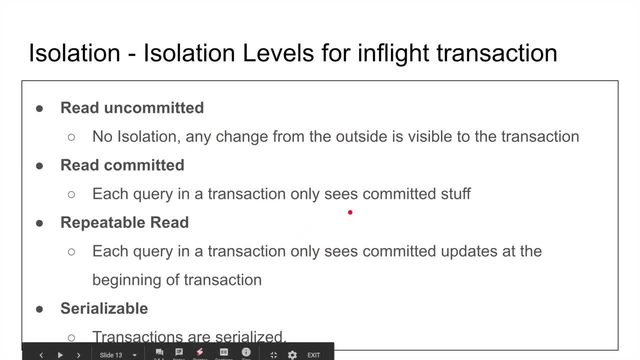 So repeatable reads, okay. So this way, I guarantee that I'm gonna read the same repeatable read, right? I'm gonna get the same read because I'm reading the same version, right? Some databases implement it as a form of a lock. 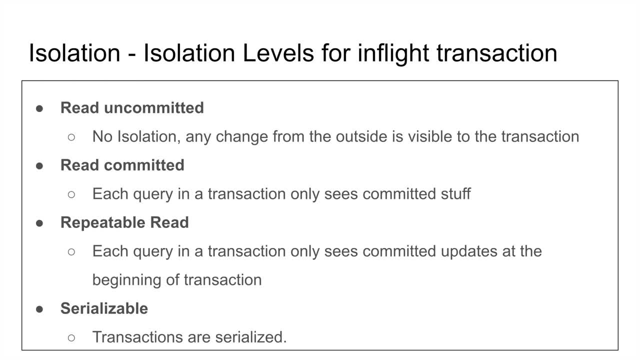 which is a little bit more expensive. okay, So you establish an exclusive lock and say, no, I am only reading this. Please, guys, don't change this. okay, Don't change it. So, once we establish an exclusive lock, 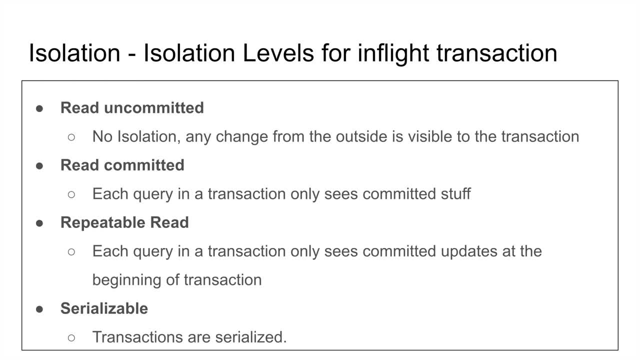 we cannot. nobody actually can or nobody can change that stuff. No, sorry, It's a flexible lock, So that's the right way to do it. okay, So the lock approach of that- another approach to another approach to implement repeatable reads- is: 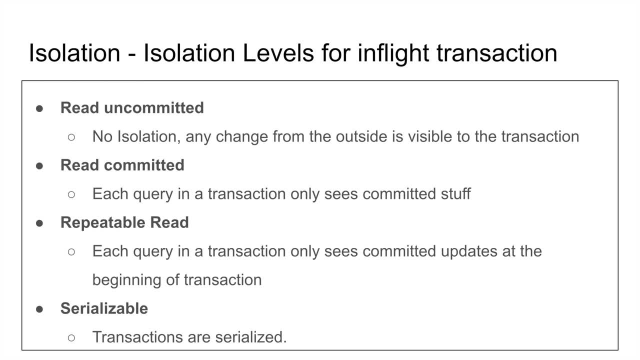 you're gonna start, you place a shared lock so you guarantee that nobody can actually change your data. because everybody that needs to edit they need to establish an exclusive lock to edit these rows. right, Then you get about what to read. 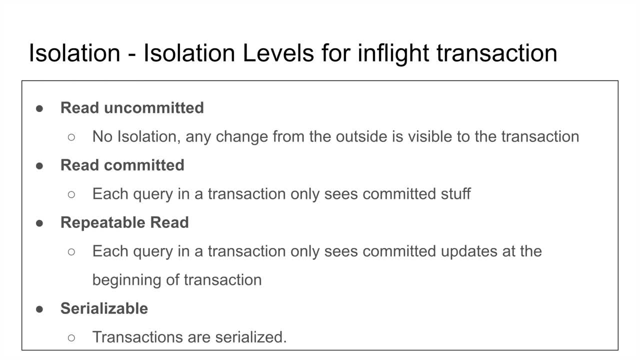 And then, once you do that, you release the shared lock. okay, So you implement some sort of a shared lock, but you just blocked people from editing, So versioning's kind of a little bit better. but there's the pros and cons for each one obviously. 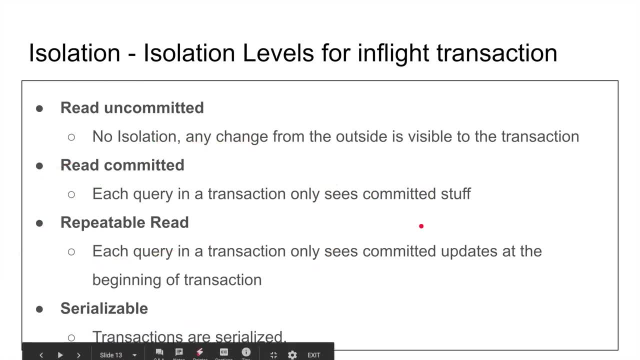 Serializable. that's the easiest way to implement and the kind of a slowest, And the performance goes down with every level of isolation. So it's like think of it as a chart. right, This is no isolation. This is the highest isolation level, okay. 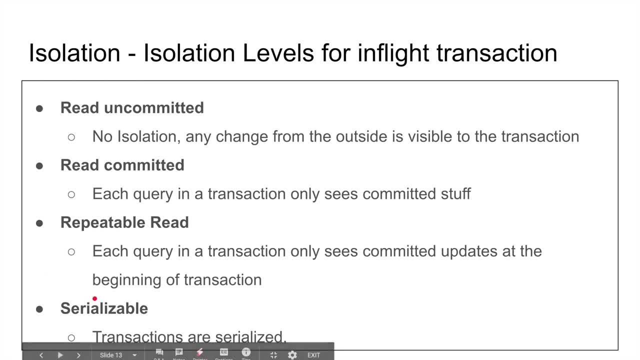 But this is the fastest thing, This is the slowest thing. The serializable is essentially, each transaction has to be serialized, right? So if you as if they are serialized almost like serialized right, So a transaction just followed by another transaction. 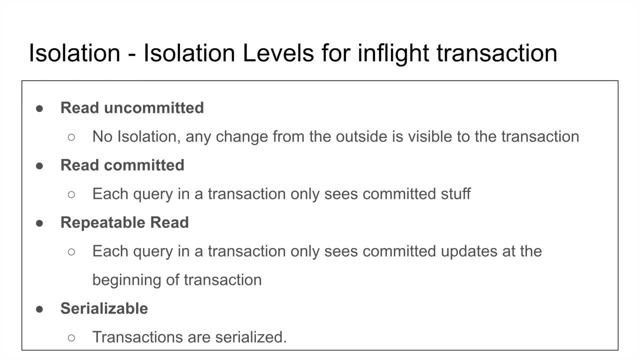 they cannot be executed in parallel. essentially They try as much as possible. The database does a little bit tricky things to execute. some of them are parallel, but most of them you can think of it as serialized right. So if you're serialized, nothing running in parallel. 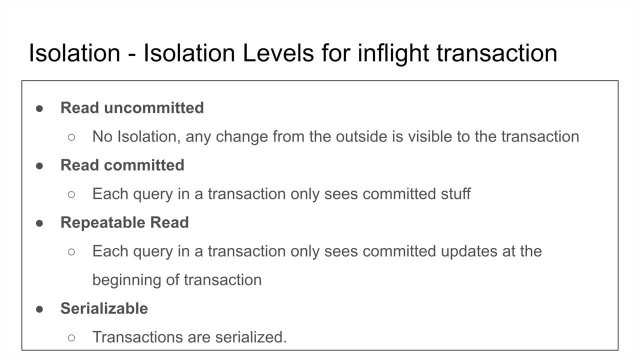 you're happy, right, This is the best thing ever. If you're nothing running parallel, then you're not gonna get in concurrency issue. You don't have isolation problems anyway. okay, So this is the best way Most of the time. 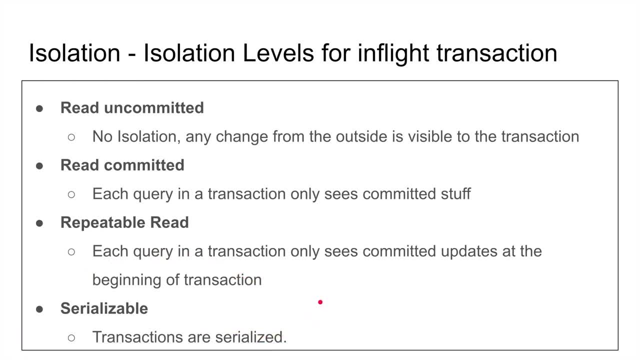 this is implemented at the application level. The application places a lock and says: guys, stop touching my stuff, I'm updating it or I'm reading it, all right, And then start reading everything and then it goes away. Okay, This is the table I was talking about from Wikipedia. 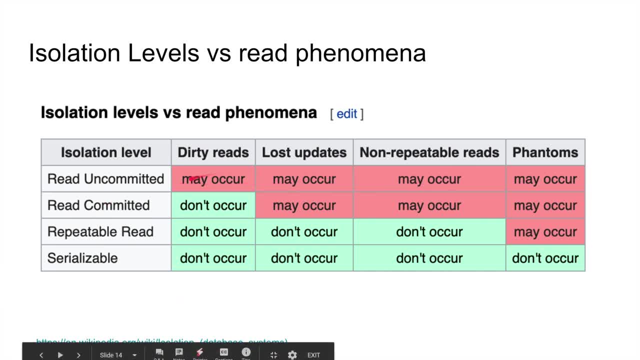 You have that read uncommitted level, All of that stuff, all this phenomenon can occur, obviously because we don't care. read uncommitted, Read anything right, Any change that happens. dirty reads, lost updates, you get non-repeatable, you get phantom reads. 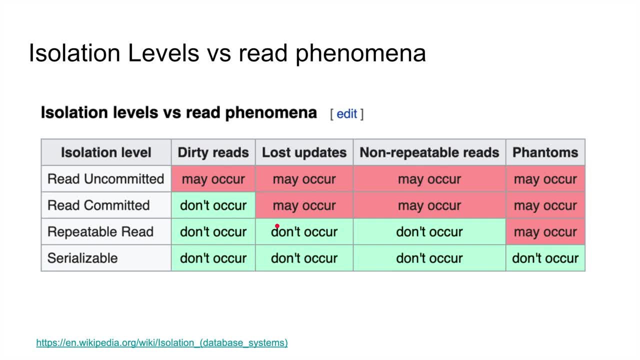 Read uncommitted. What are we gonna do is essentially read only the committed stuff. So you're not gonna get dirty reads. You know that because you're reading only committed stuff. but you're gonna get non-repeatable reads because each query is getting the new committed stuff right. 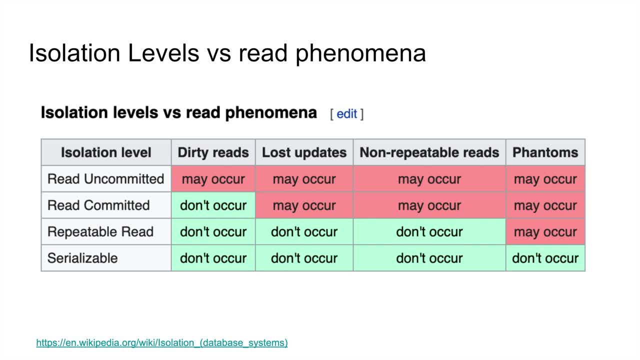 So if you queried at point the first query of the transaction and then you turn around and queried again between those two queries, someone might change the value and committed it. So you're reading the committed value, but it changed. So it's non-repeatable and that might not be desirable. 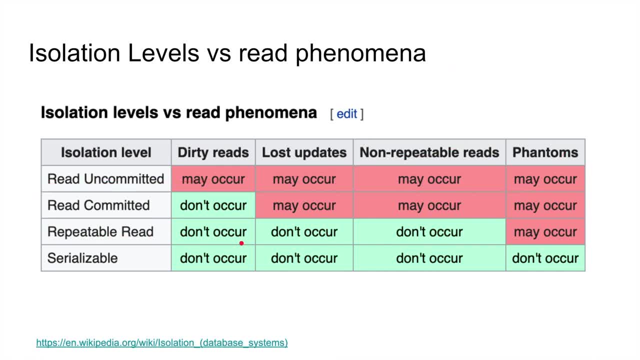 Obviously, you might get phantoms as well. Repeatable read: You're not gonna get dirty reads because we're reading only committed stuff. but in addition of that, we're only reading committed stuff at the beginning of transaction, So you're not gonna get a non-repeatable reads. 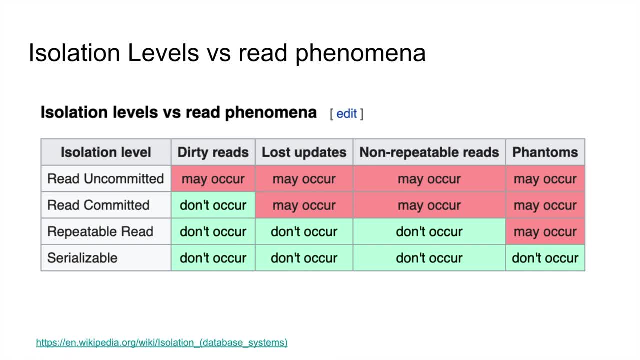 All of your reads are repeatable because you're reading the same version of the database at the start of the transaction, or the database will force you to places lock and then will only read the stuff at the beginning. okay, So that's essentially a non-repeatable read. 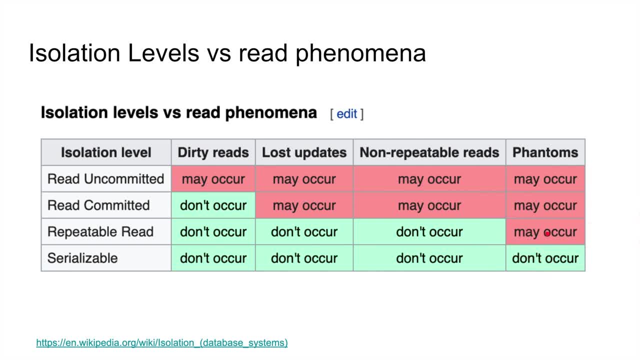 And, but phantoms still can't accurate as a result, because you cannot control new rows. You can only controls what you can only control: rows that you can lock. right, And this is debatable. With versioning, you actually can get away with it, right. 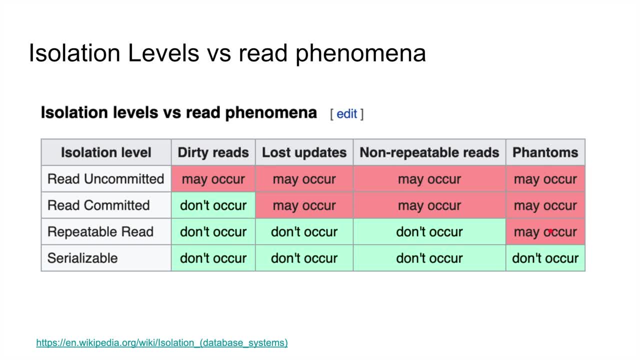 So this table is not entirely accurate. If you implemented versioning with more repeatable reads, you can- actually you might- get away with repeatable reads right, If you implement the versioning. I think RocksDB and the Facebook data storage engine. 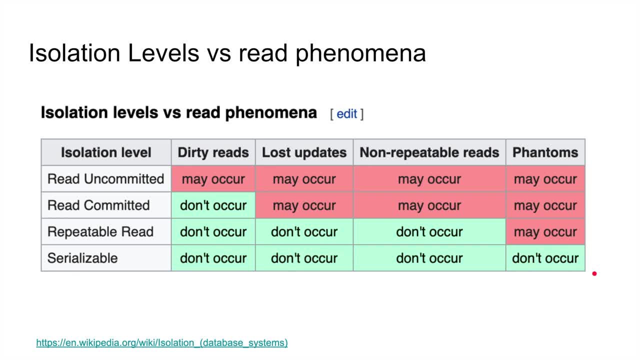 implements that versioning Serializable. best thing ever. I'm not gonna say best thing ever, But if you serialize your transaction you're not gonna get any of that stuff right? You are guaranteed that nobody touches anything unless they have a lock, right? 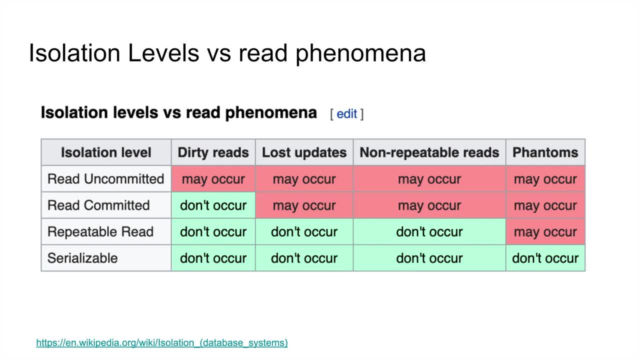 So you start the transaction, you place the shared lock right And if someone wanna implement an exclusive lock, they will get an error because there are shared lock, there are read locks. So, and we talk about shared lock and read locks- 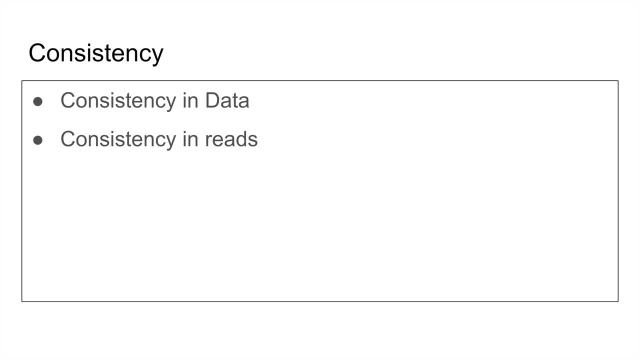 I'm gonna reference the video there, guys, All right. consistency, guys, All right. so I really needed to talk about authenticity and isolation first, to talk about consistency, right, Although consistency is the second property or an asset, right, And the reason is: 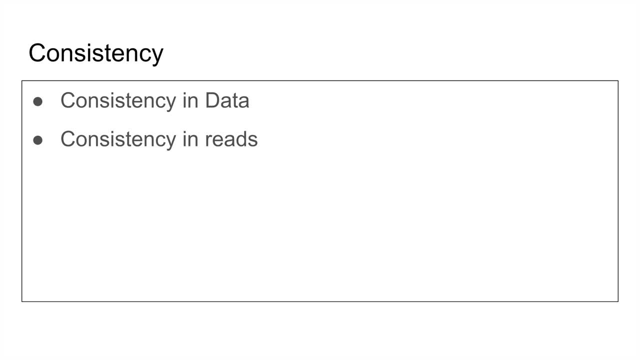 atomicity and isolation leads to consistency. in my opinion, right, And the way I see it- there are two types of consistency, the way I see it here, And the first one is consistency in your data And the second one is consistency in reading the data. 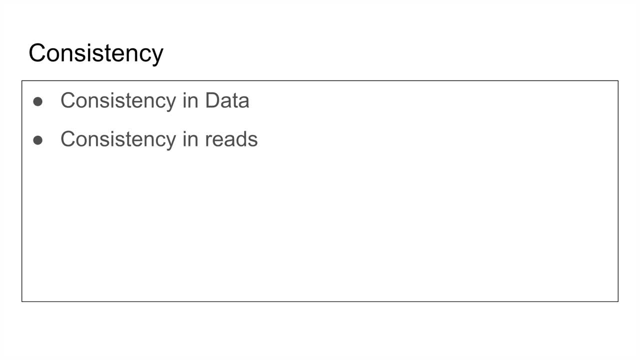 And let's talk about each one of them. And let's talk about which one of those the NoSQL guys came and tried to to improve upon. okay, And try to kind of be relaxed here. Consistency in data. Consistency in data is essentially 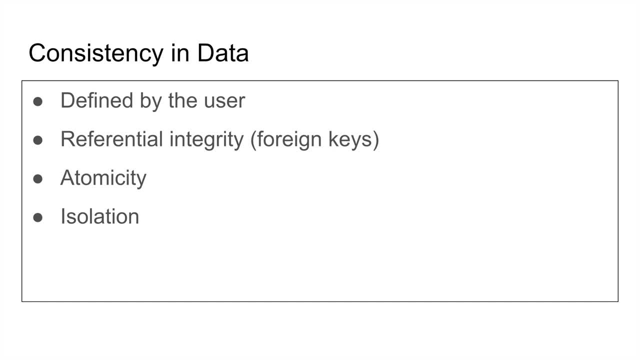 is defined by the user. It's something that the user defines in their table schema. It says, hey, this view and this view should be consistent. Like, say, the sum of the money in this table should equal the sum of all the balances or the number of likes in this picture. 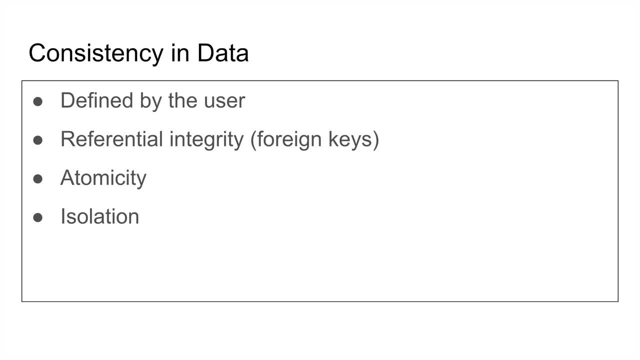 Should equal the number of the users who actually liked that picture. So this is a consistent view that the user defines. okay, Usually it's enforced by referential integrity, like foreign keys and primary keys, So you ensure consistency in your data, And it's also ensured by atomicity and isolation. 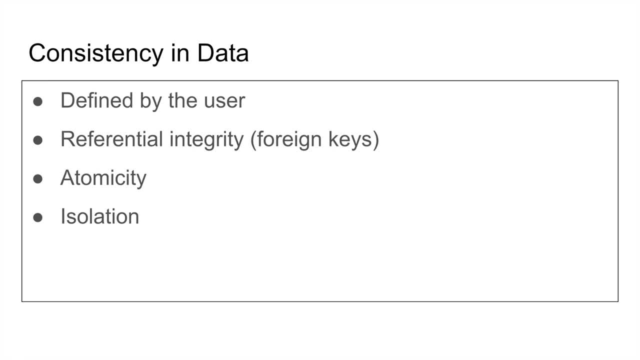 We saw that. We remember when we got the blue screen of death in the middle right. We just bleh, lost my data right Just went away And I got an inconsistent balance sheet as a result. We got 900 and 500,. 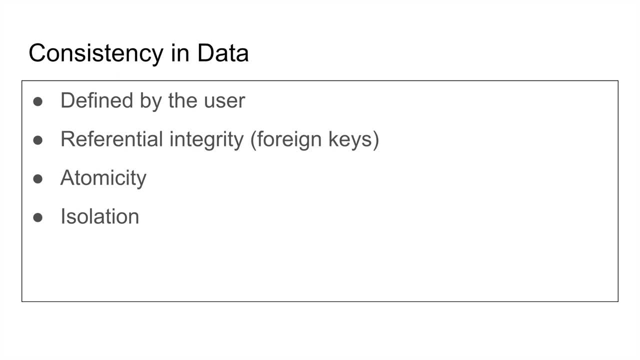 where 100 just went away in the thin air. okay, So lack of atomicity leads to inconsistency in your data. Okay, Isolation- Do I need to say anything? We saw all that stuff with isolation right, Giving all this false reports. 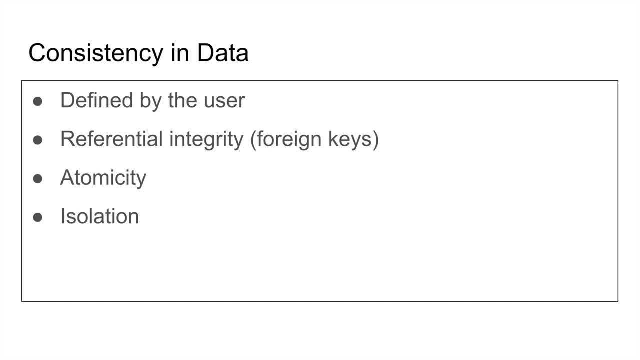 as a result of lack of isolation. right Being the moment, people are changing my product sales while I'm reading this data, I'm gonna get bad results. I'm gonna get an inconsistent result. okay, Although my product says the sum is 130,. 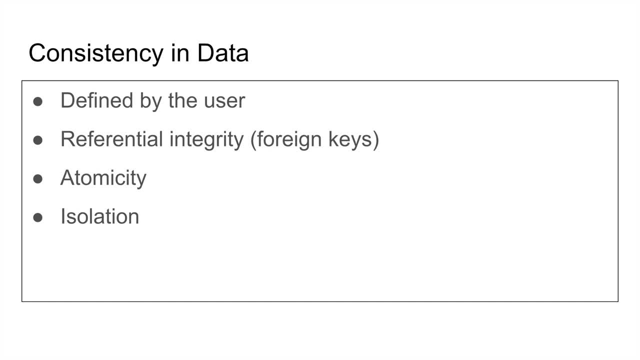 I can see it, I can sum it, but the actual total is saying 155.. That's bad, okay. So lack of isolation leads to inconsistency. It's up to you as a user if you can handle, if you're okay with that inconsistency or not. 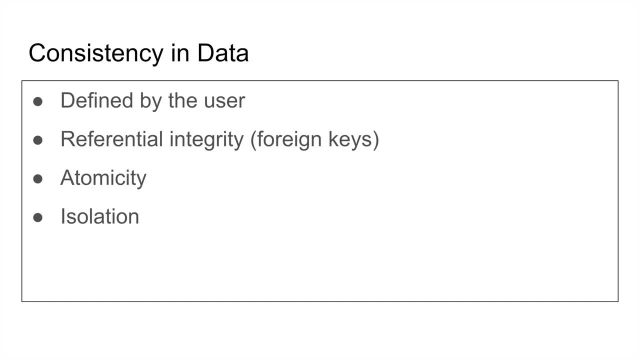 Sometimes it leads to corruption inconsistency. If you're not happy with that like a bank transaction, you cannot probably be happy with that Product sales- probably not. That's bad. right Pictures and likes. eh, we're gonna show that example. 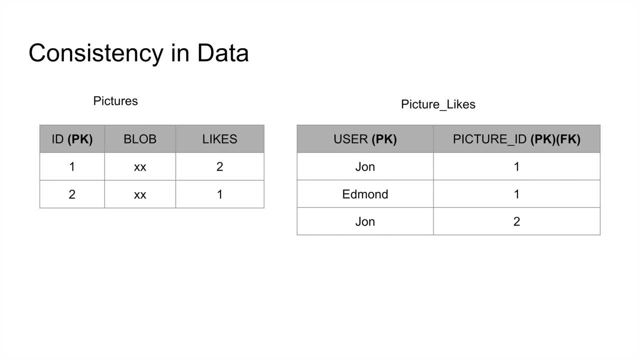 See, like this is an example, right, Where consistency in my data is really not a big deal, right, Like we have two pictures here. This is a blob of the picture. Let's say this is an Instagram implementation. We have a blob. 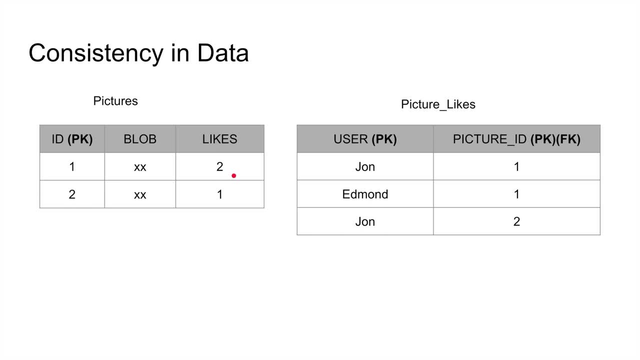 Of the picture and we have the number of likes. right? Hussein might say Hussein. why are you adding a field called likes? What is that okay? Why don't you just query this table and just get the number of likes? 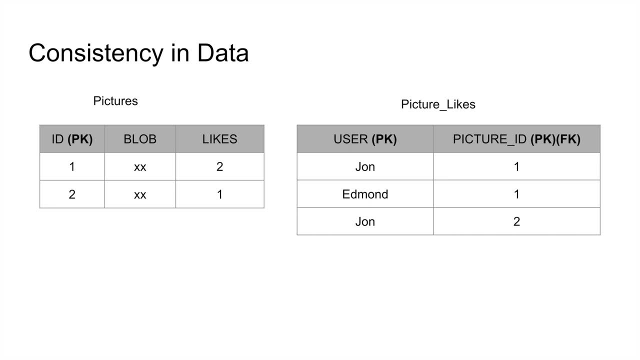 Performance is the best Short answer for this right. So you would add a likes field here which will contain the total number of likes in this picture that this picture got. And there's another table called picture like, which includes like: hey. 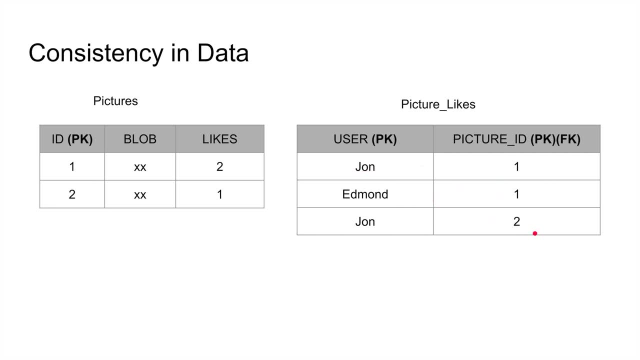 John liked picture number one, Edmond liked picture number one, John liked picture number two. So if you sum this right, Picture number one got two likes from John and Edmond. That's correct. And then picture two got one like. 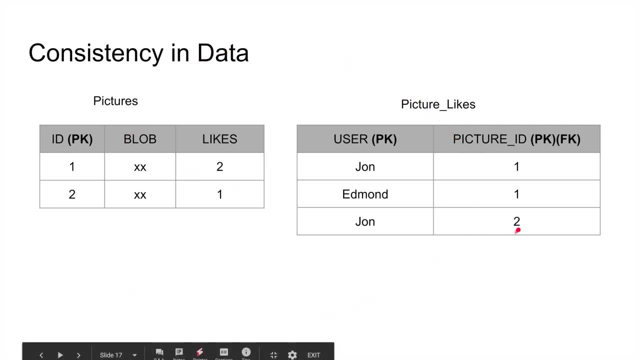 It's one from John, So that's a consistent view. But if you saw like, for example, this is four and this view doesn't represent it. that's an inconsistent view. It's up to you if you're happy with that inconsistency or not. 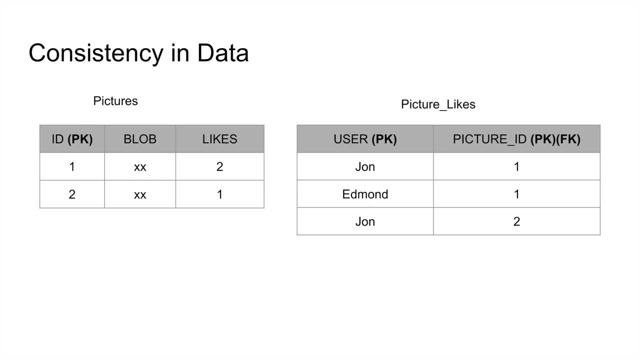 And that's a very critical question Because, based on that, you can adjust the performance, You can adjust the consistency, You can adjust scalability, You can adjust isolation right. Based on what can you give up as an engineer, As a software engineer? 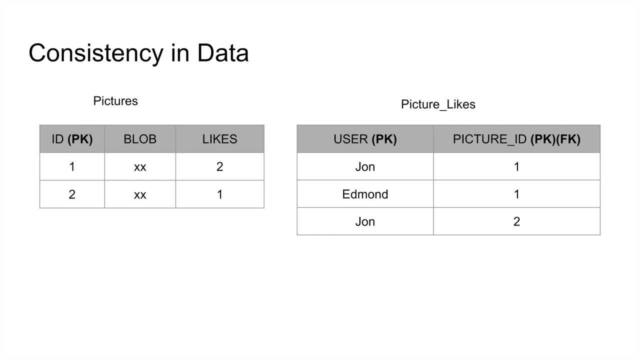 you really, guys, need to think about every single aspect of that. What can you give up? That's why you have to understand the requirements and then ask yourself: what can you give up? You're telling me that Instagram, Instagram and Facebook instagram if, if kylie jenner gets like 5 million likes on a picture, 5 million and 32 likes if i? 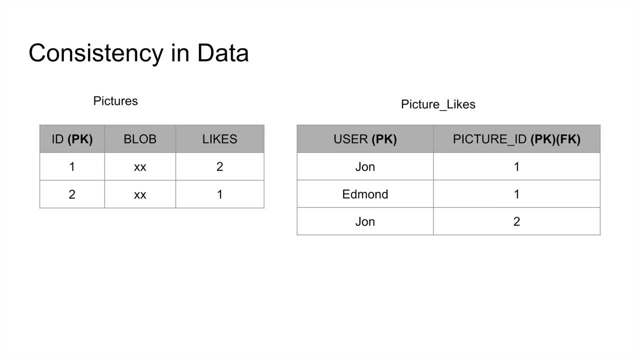 clicked on that and view the 5 million. are you telling me they're gonna match? i'm betting everything you want. they are not matching this. this is impossible to get in consistent view on this right. and they don't care, because nobody's gonna fiddle through 5 million users anyway. so 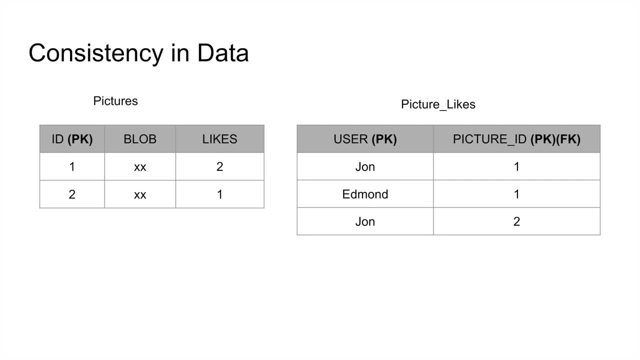 they can give you an approximate number and they can be off. there's those two views can be off by even hundred thousand. youtube is the same subscribers, right, do you think? why do you think youtube is showing you like my subscriber is 6k or 6.2k? because they cannot guarantee you. 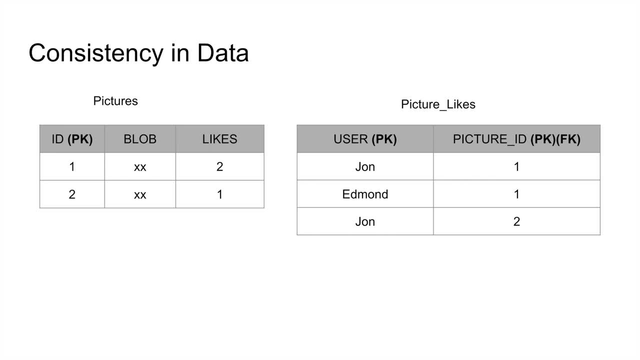 that i have exactly 6032 subscribers. okay, or 23, or even. uh, pewdiepie right, he has like one, now one, almost 95 million subscribers. that number is not exactly accurate to the actual number of subscribers that he actually got. it's an approximation. because they cannot, they decided. 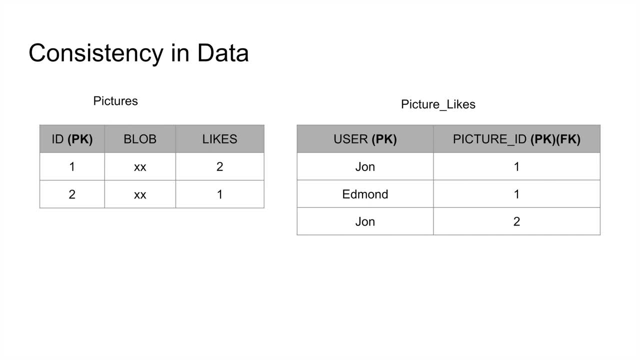 it's not important to maintain the consistency of this thing. because why? first, because nobody's going through 99 million subscribers, so they are preferring performance over this consistency. sorry about guys, sorry sorry about that going to a tangent, but it's- i think it's. it's critical to this let's talk about. 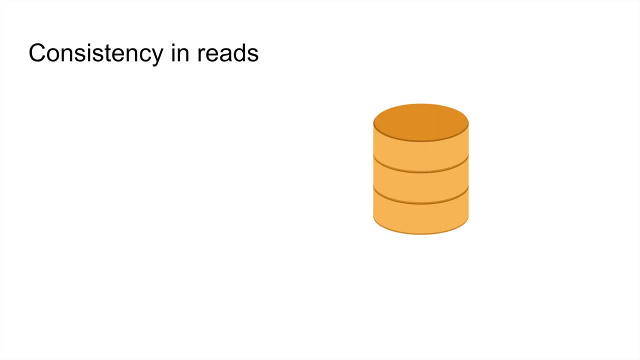 the other cost concept of this, consisting in data. sometimes it matters, sometimes it doesn't. consistency: consistency and reads: same thing. sometimes it doesn't, sometimes it matter, so we'll think about that. now, consistency in reads is very interesting and, uh, what it means is like, if i update something, if a transaction updates something, i'm going to update something and i'm 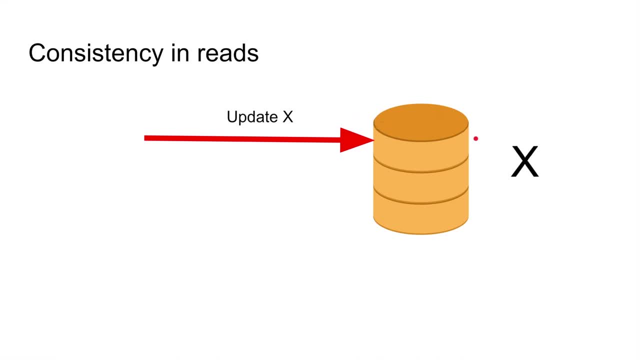 going to update something and i'm going to update: um, let's say, a value x and that x gets persistent, and then another transaction start reading that it better get the value x. hussein, what are you saying? that's obviously tough freaking duh, right? obviously it has to get the same value, but not. 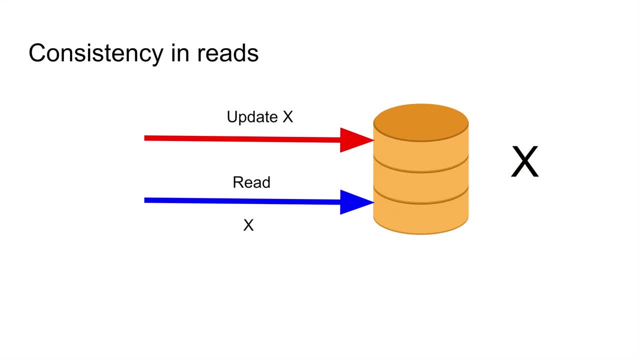 necessarily. we're going to talk about the concept of eventual consistency here. so that's inconsistent read. if i committed something, can you transactionally get value? if that's inconsistent read, that's not consistent, and so i have to make a comparison- that's interesting as well- about that. okay, let's. 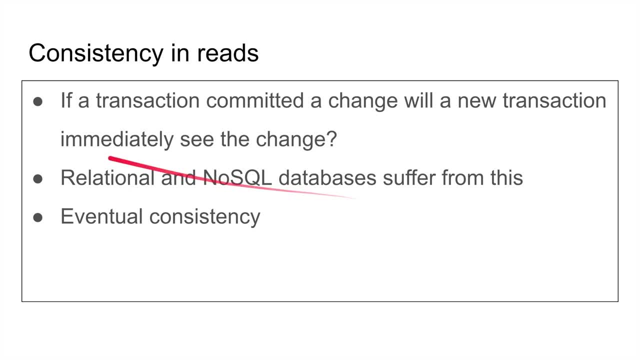 see what we're gonna do, how to deal with that. first let's go ahead and say: if the transaction gets, see it immediately. okay. and here's the thing. this move type of consistency is unavailable on both relational and no sequel databases is a big statement here. okay, both databases suffers from this consistency. okay, including Oracle. 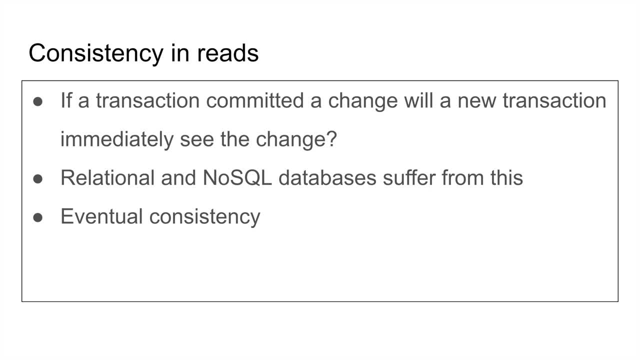 including Postgres, including my sequel, those that is are not consistent and reads. and let me explain here: when you have a one server and you're committed something to it and you read from that one server, life is good, right, life is perfect because you have one freaking server. but the moment you start adding 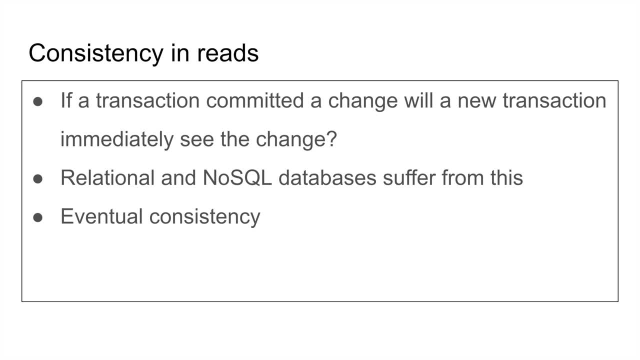 other server. let's click about. this is positive. oh, my sequel, right. what are you gonna do, essentially is you're gonna have one server and you create in a replica of that server, and that is like even one way, or a like our two-way replicants is gonna start pumping data to the replica, right? 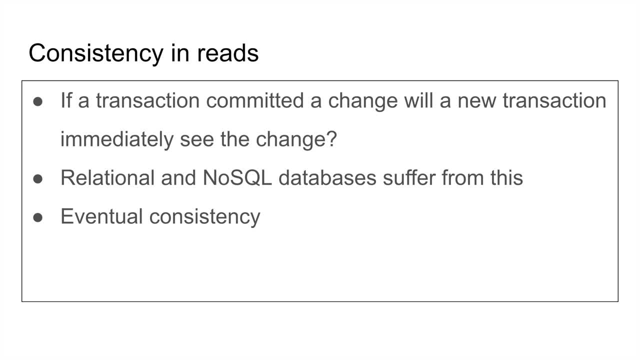 and now obviously you need to add multiple replicas for horizontal scalability, right? you cannot serve 7 million people of one database, right? data YouTube started doing that with one database and they scaled it up to multiple and they implemented now fit test, which is this new fancy stuff on? 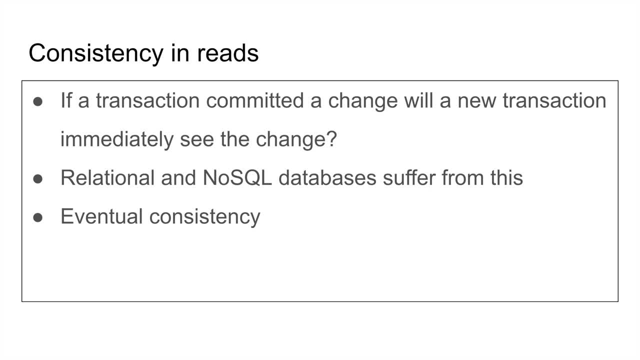 top of my sequel that that gives you, like sharding, on-the-fly, sharding, allowed stuff. we're gonna talk about another video, but essentially, the moment you break things up into these replicas, into this essentially the other databases, right, this secondary databases, the follower, leader of follower nodes, right now when you start doing that, you 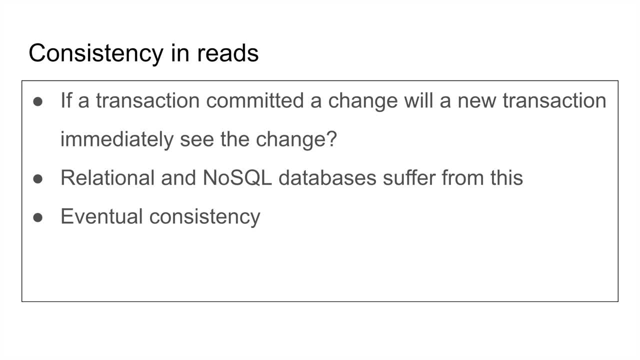 are inconsistencer. you will become inconsistent because you will write your to the primary node and someone else reads from the secondary node. the secondary node takes time to get the value propagated. there is networking going on, there is delays, latency, until the secondary node gets the new value. so you're gonna get an old value, my friend. you're gonna get an old. 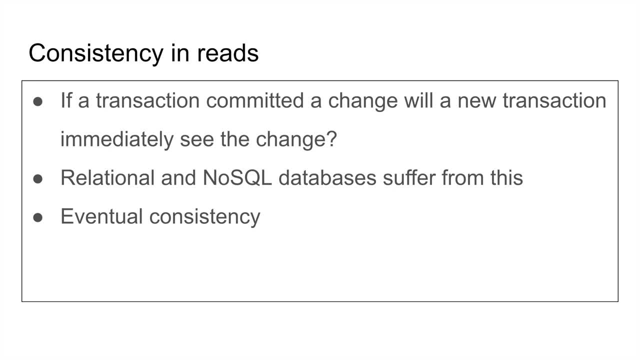 value: right and that is inconsistency. so this problem and a lot of people get this wrong. inconsistency so the relational database is inconsistent in reads- right, the moment you start breaking them into horizontal scalability, multiple servers, you're gonna get inconsistency right. so they are consistent when there is one big nice server- right, the moment you break them. 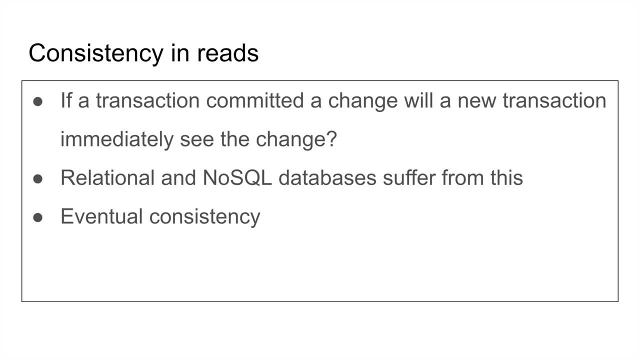 they are inconsistent reads. you're gonna read it, but someone we're gonna read an old value and it's up to you now as an engineer: are you happy with this old value? if you get an slightly older subscriber count, okay, that's completely fine if your video the latest view and that's what like. 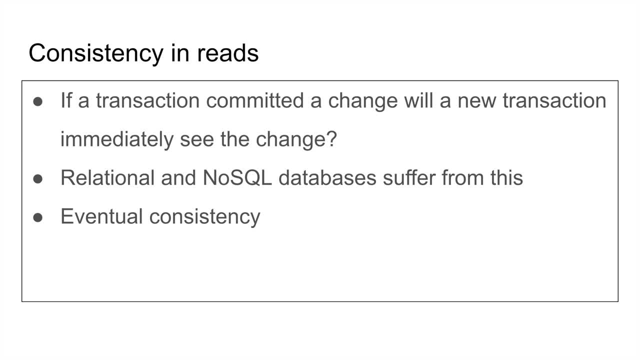 YouTube does right, is their money, servers and all these rights going to multiple databases and then they eventually sink into the database. and then they eventually sink into the database and then back into one big server, one big database, right, and then if you read, if I'm reading that view: 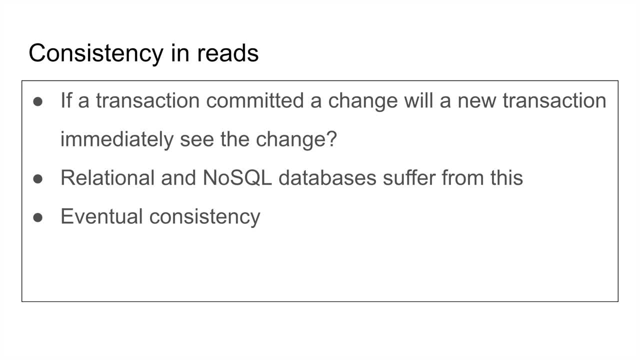 versus someone from Germany versus someone from Japan. reading that same video, we're gonna get different results. because we're reading different replicas, we're eating from different follower nodes and that's okay, right, sometimes that's okay, sometimes it's not. so now there are a bunch of 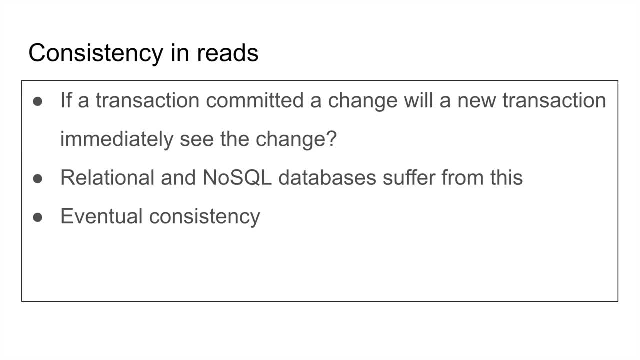 people who say: you know what? we don't want to enforce that thing. this is all the stuff you guys are doing silly. this acid thing is silly. and the fact that scaling relational databases has been always hard right, because was designed in the 70s to be a one big. 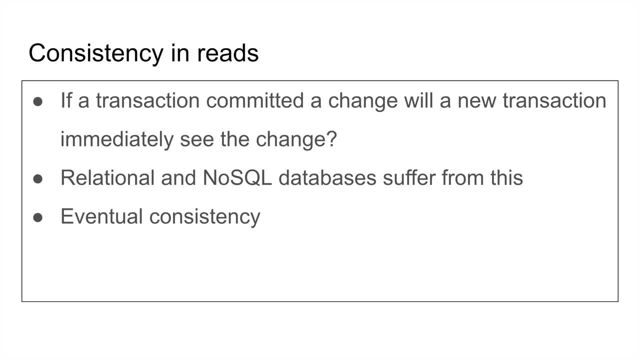 beefy machine. right, one big beefy server, the database is there and that's it. right. in this era, those guys said: okay, you know what, I'm gonna give up consistency, because you guys are already. you don't have consistency. you're gonna give up consistency. you're gonna give up consistency, you're. 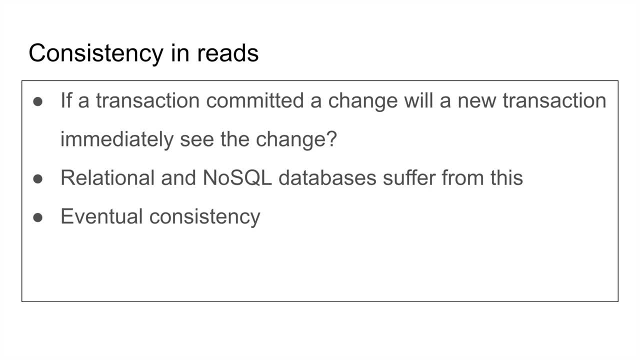 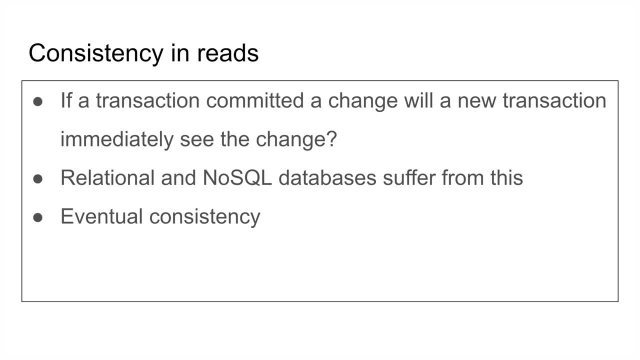 gonna scale horizontally, we're gonna add a bunch of other servers on the size and then just stick. yet we're gonna- we're gonna start charding, doing all these things and distributed manner, okay. so that's essentially what they did, and there was thus the nose sequel. databases came into picture. 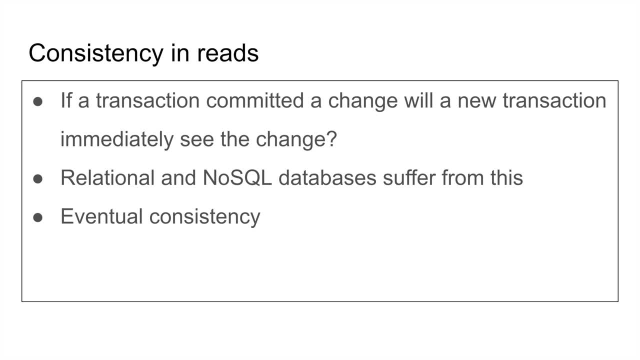 Okay, so they give up consistency or on favor of scalability, which the relational databases are really really hard to do, right? Relational databases where you have to implement the follower node and leader node and they start replicating, pumping changes right. 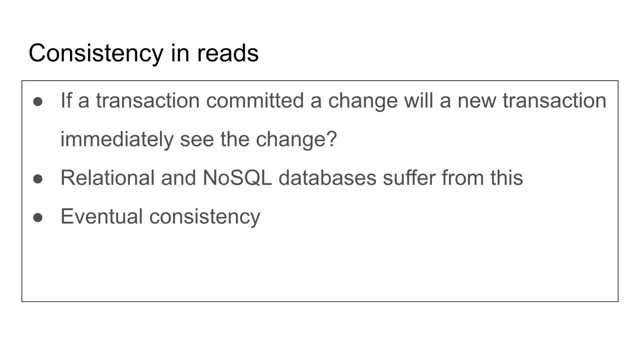 And the NoSQL one gives you a scalability. You can add just nodes and they will scale nicely. Okay, but if you're looking for isolation and all that fancy stuff, you're not going to get it, obviously right. Okay, you're not going to get all these properties off of this. 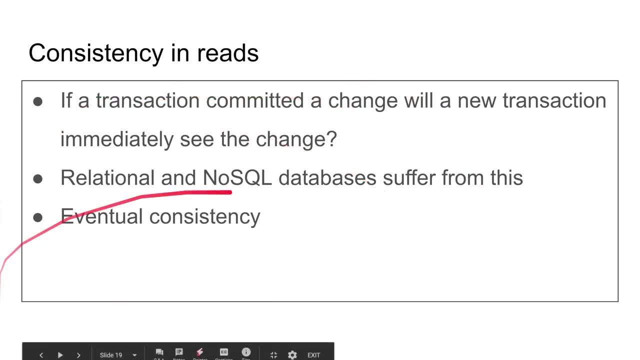 You will get this new concept called eventual consistency, which is, to me, is just a marketing term. Okay, eventually, everything is eventually consistent, duh, Okay. so it's like if you read the value, you get an old value. If you wait a little bit, you're going to get the 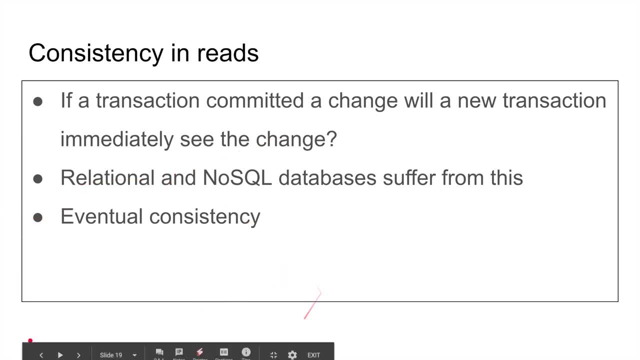 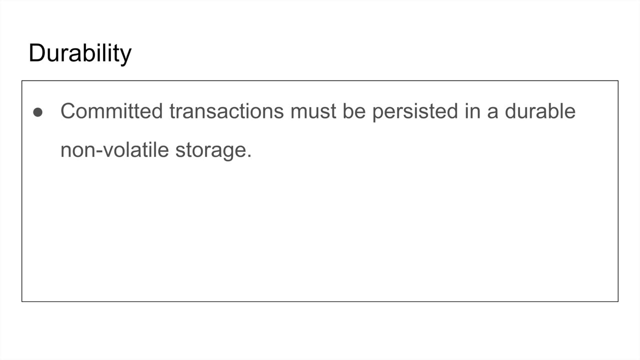 the latest value, essentially right. So to me, eventual consistency: both the relational databases and non-relational databases suffer from this. okay, eventual consistency, Durability: committed transactions must be persisted in a durable, non-volatile storage. So that's what it means. 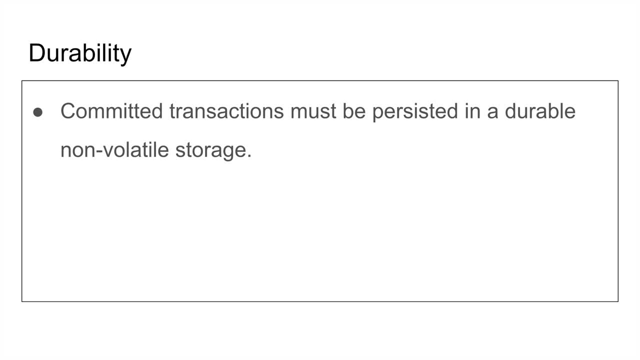 If I write and committed a transaction, it better stay there when it's when I lost power. If I committed a transaction and I lost power and database shut down. if I restarted, the value better be there. That's what durable, durable means, right. 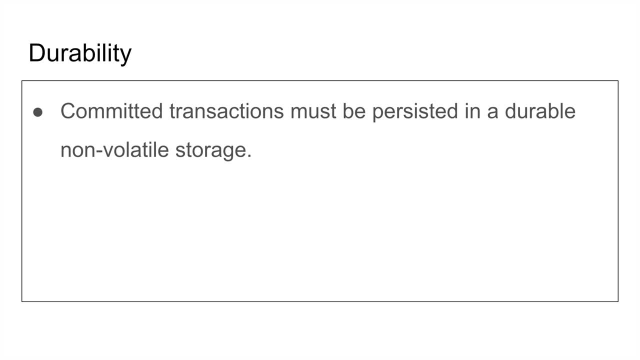 So Redis, for example, is not a durable database, It's an in-memory database. Memcached is an in-memory database. It's not durable And it's up to you. If you're caching stuff, you're just doing, doing stuff for caching. 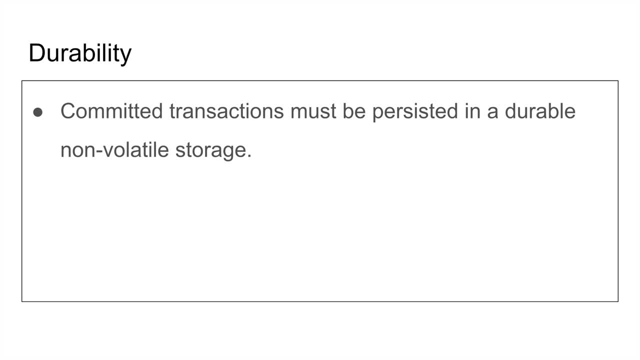 you might really don't care about being durable, right? So a lot of databases took these four properties and just starting hacking one of them out and then creating, creating a brand new database out of it. So Redis took the durability out and they just created this in-memory database thing. 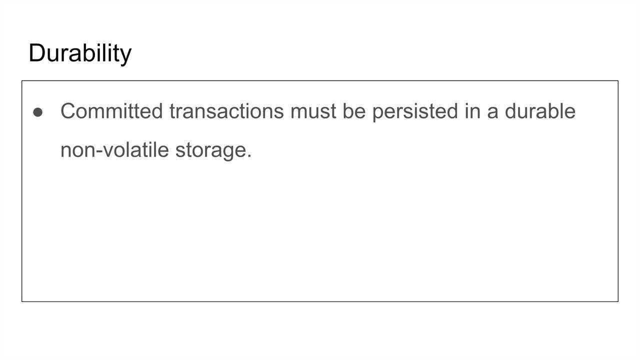 They have, I think, persistence. I didn't work very closely with Redis, but the in-memory they have persistence model. I think Cassandra and MongoDB decided to say you know what? I don't need consistency. I'm going to give you consistency. 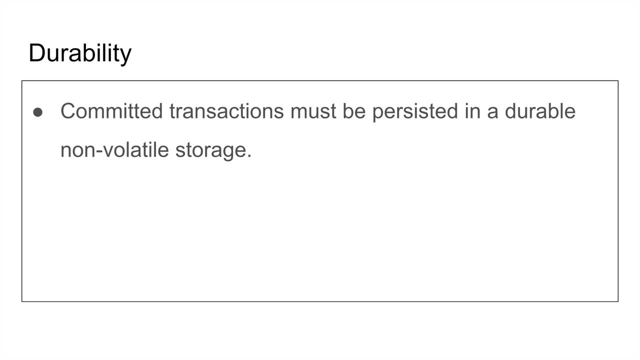 when you write your query, right, But you don't need consistency and you don't have a schema to begin with, right? This is there's a lot right. There's a lot of things that got relaxed, not only just the consistency part of it. 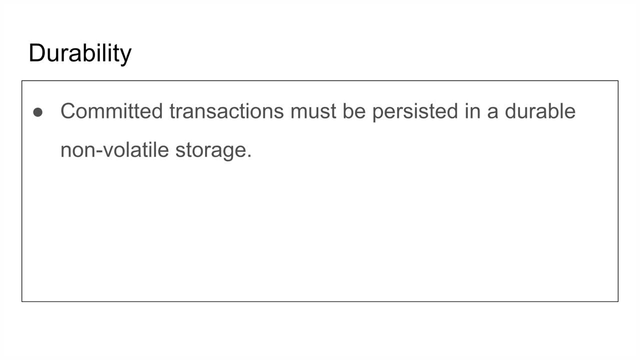 So there's no schema, no referential integrity, you don't get indexes, secondary indexes, all that stuff. You don't get any of that okay, So really that's probably another topic, NoSQL versus SQL. but yeah, that's it guys. 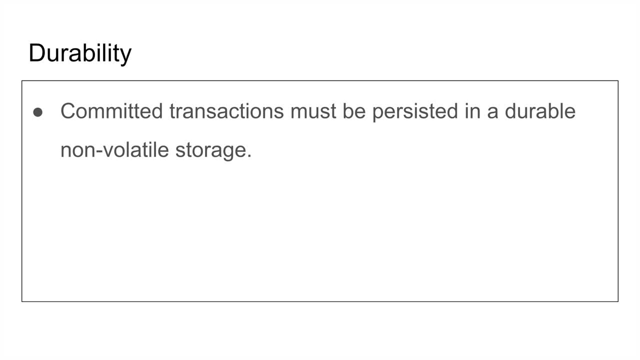 A long video. you made it. Thank you so much for watching until the end. If you reached it here, leave a comment at the end. like this video. if you like it, share it with your friend. It's almost like a course.